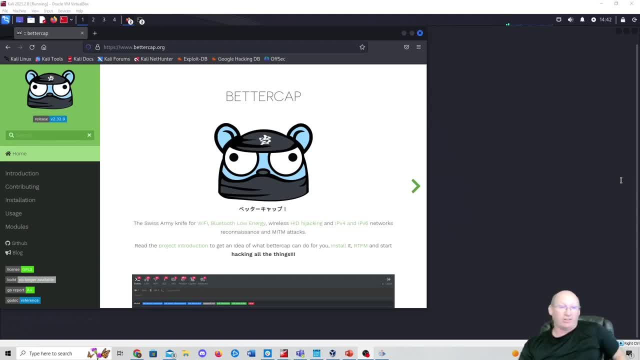 and they didn't give you permission, then you could be held liable under the Computer Fraud and Abuse Act. So make sure that you understand the confines in which we're operating this lab in. Again, if you go outside those confines you could face some pretty hefty fines and jail time. 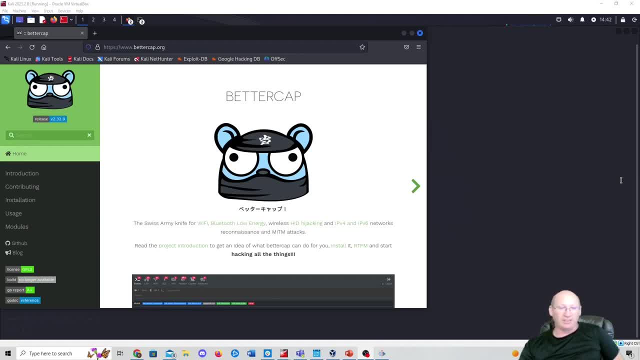 So I want to warn you once again: we only do these little labs that I'm providing you inside of a virtual environment, inside of a sandboxed environment in which you own the assets. With that said, let's get started. All right, so this lab is going to be a little bit different. We're going to do address resolution. 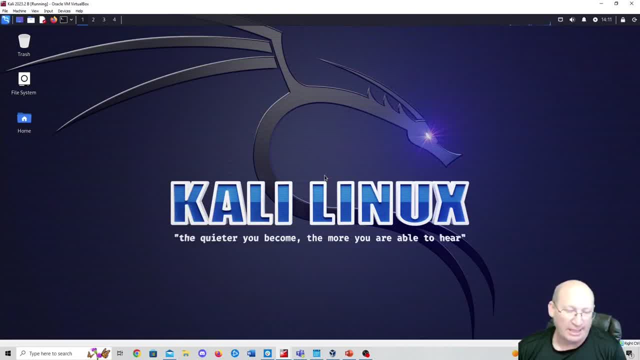 protocol poisoning or ARP poisoning, and that has to be done inside an environment that utilizes THCP. If you've seen through my other videos, you probably realize that my home lab is usually set up with a static IP address as opposed to a dynamic IP address, so it really wouldn't work in that environment. 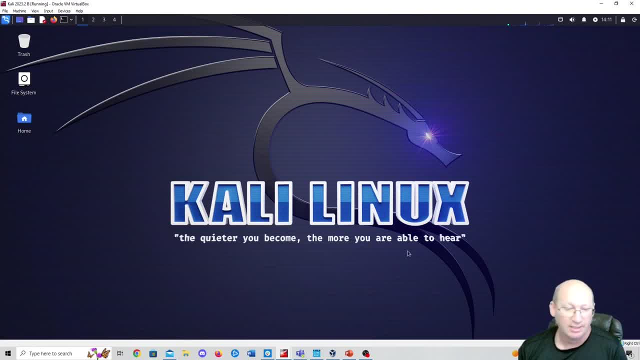 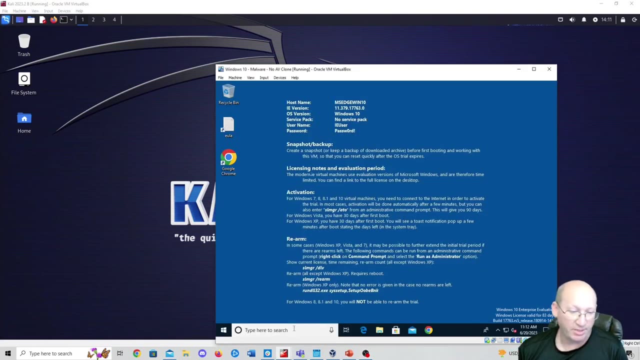 So in this case we've decided to use Kali Linux using DHCP, and then I set up a secondary Windows system utilizing DHCP as well. so it's outside of our normal lab environment. So let's just get into it and then we'll go from there. So you can see, here is my Windows system and I'm going to go into the. 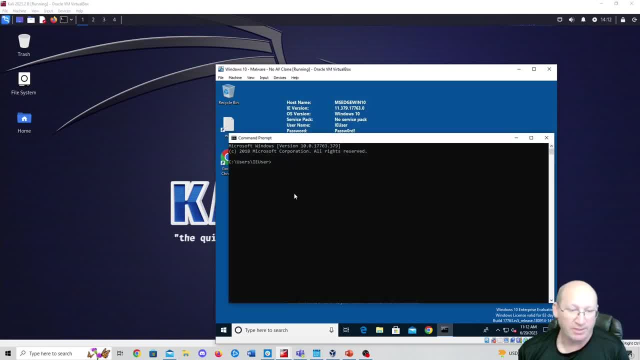 command line, the CLI. To get there, I type in CMD under this little point right here, just CMD, and that'll get me to the command prompt. and that's what I'm looking for, And we're going to take advantage of ARP address resolution protocol. So first I want to point out 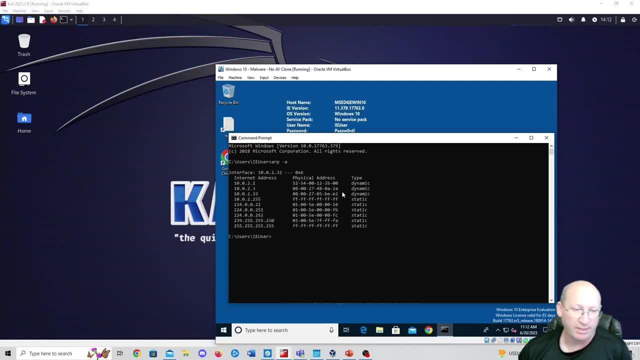 what ARP is. So we're going to do an ARP-A, and this will give me all the devices on my current network that are utilizing that same atmosphere, And I can do the same thing for my Linux as well If I go to terminal over here. I'm going to do. 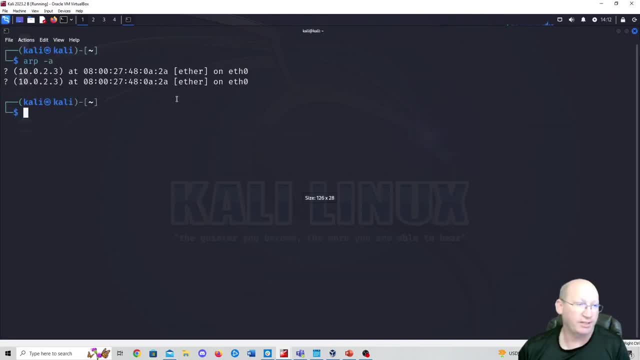 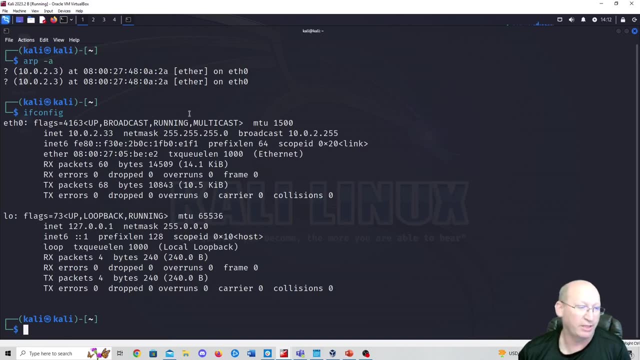 ARP-A. Let me blow this up a little bit for you. This machine is only showing itself. It's not even showing any other. it's not even showing itself, to be honest. It's just showing a .3.. So we'll do a quick inmap. I'm going to do a switch SN and then 10.0.2.0.. No, that's not working. 10.0.2.0. 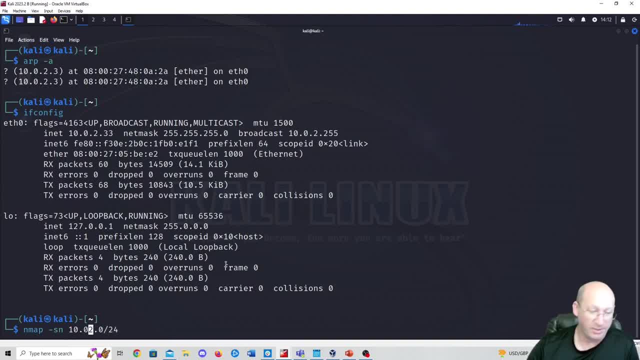 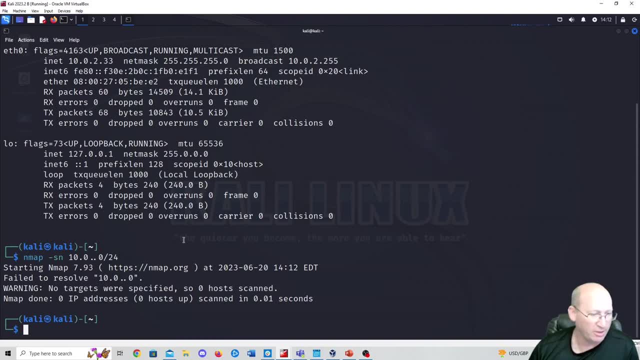 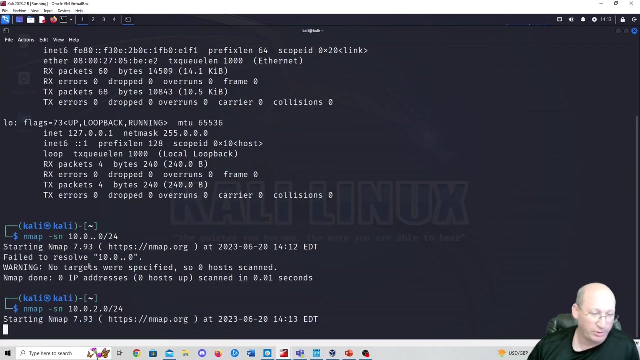 forward slash 24.. This is going to be a ping sweep across the board for that network, which will pretty much hit all the devices that are currently on this network. And obviously I screwed up a time, Just a typo right there- This 10.0.2.0.0.0,. there we go: .0.0 for 24.. That'll ping all the devices on the network, which will 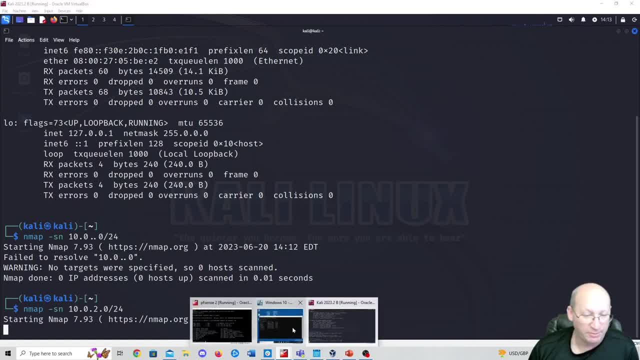 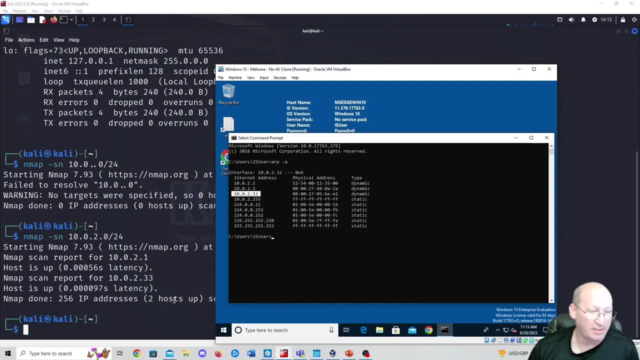 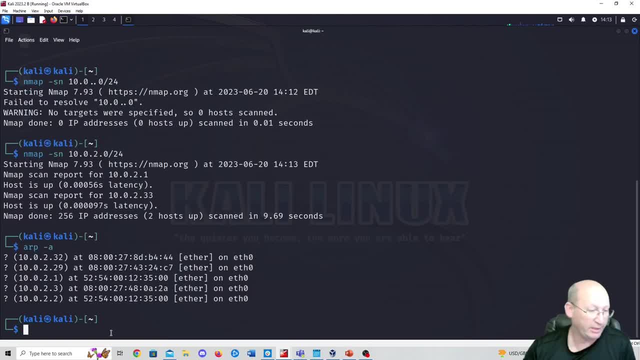 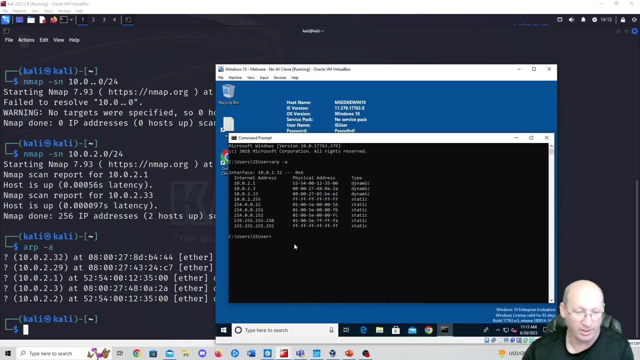 not even seeing those other devices. yet let me do an r dash a here we go. so we got 32, 29, 1, 3 and 2. 29 is my firewall, which i have working right now, and where is my windows box? let's see this ip. 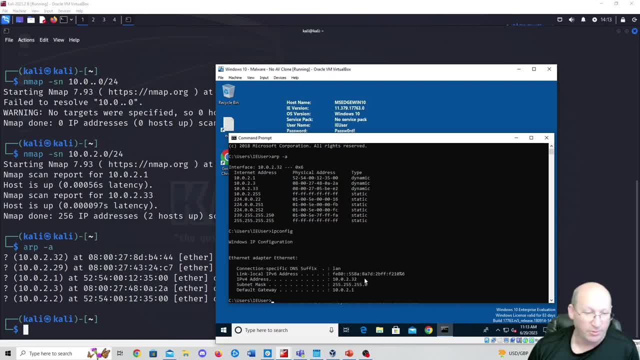 config, ip config. we're operating on 32, so it's showing 32 right here, which is where we want to all right. so i want you to pay attention to this, right here under the windows box. i want to kind of highlight this. right here we're under uh 33. if you look at this physical address, that mac. 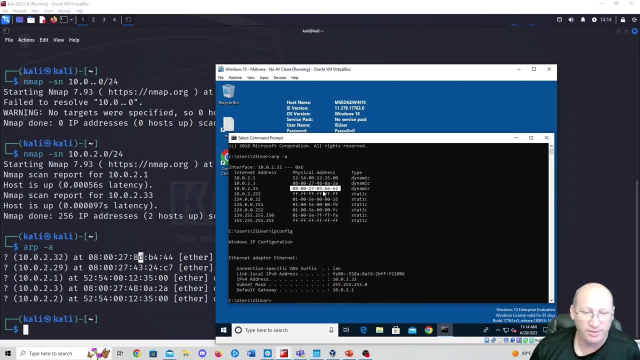 address. right there we can see it's on 08002705be-02. that mac address is where our linux box is, and then you can see our 2.1. that's our gateway right. that's our default gateway and virtualbox uses just like a regular system. 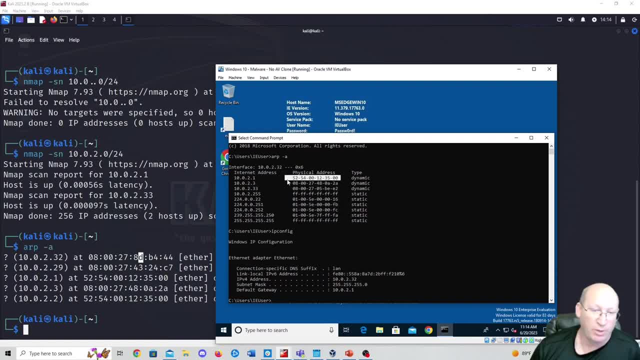 this would be your router or, uh, your exit point of the network. this is our default gateway, and you can see that physical address right here, that mac address: 5254001235.00. so what we're going to do is we're going to trick the windows machine into diverting all of its traffic through. 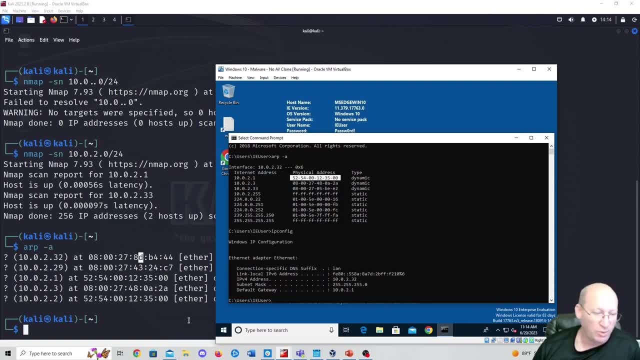 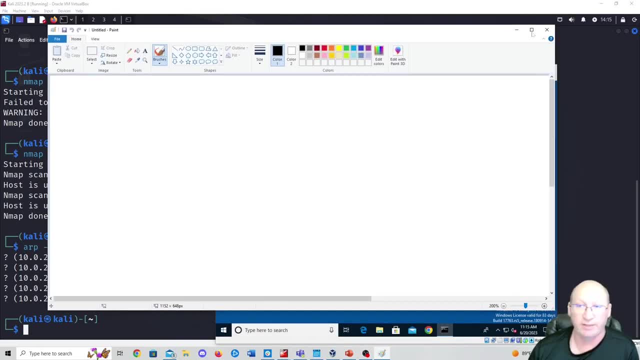 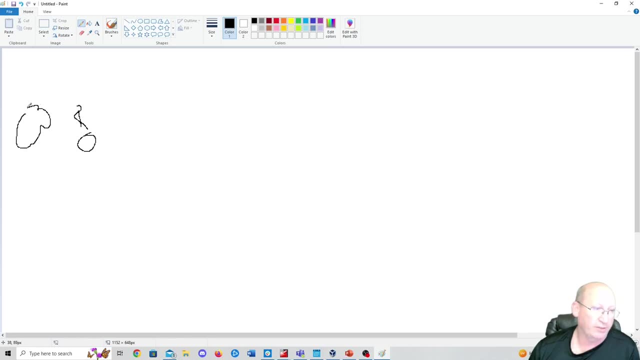 the cali box in order to get outside the network. so so let me throw this up on paint real quick and show you what i'm talking about. all right, let's let's kind of dive into this in a normal network. right, we've got our router right here. this is our router. we have our internet over here. i know my. 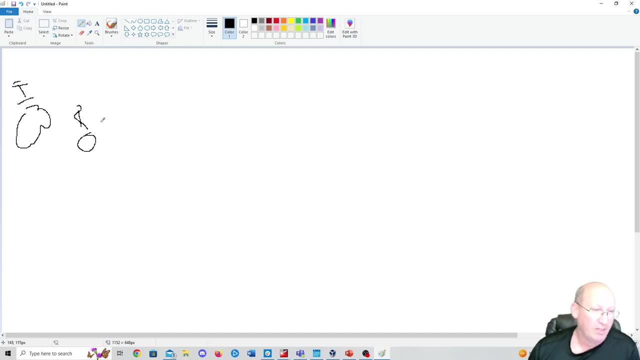 paint program just doesn't work well. my drawing skills suck right, i get it, it's okay. uh, this is going to be our 10.0.2.1, right here. this is our default gateway. this is our router. this is where everything exits out and goes to the internet over this way. on this side, we have two boxes. we have 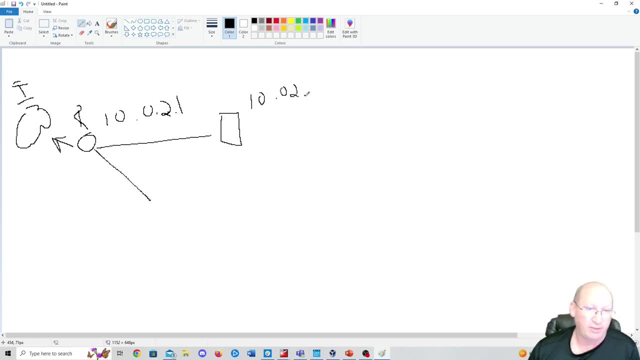 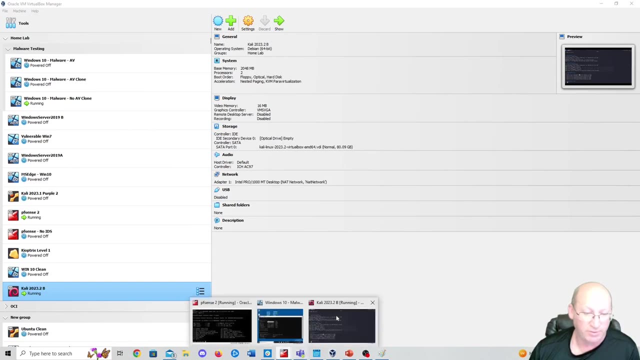 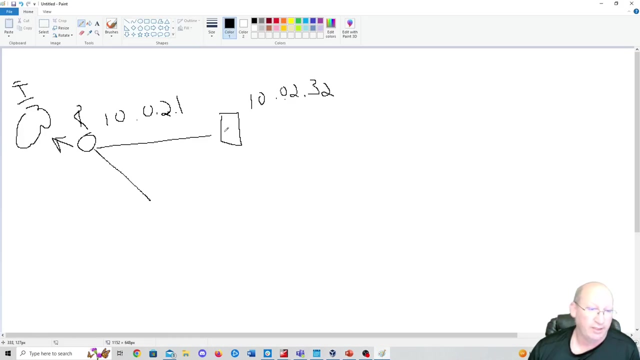 our windows machine. right here, we're at 10.0.2.. what are we at for windows? i think it's 31 in my mistake. i'm probably wrong with this. i'm probably wrong with this. i'm probably wrong with this. let's find out. oops, let me throw this over here. windows box is on 32, so 32 and that's windows. 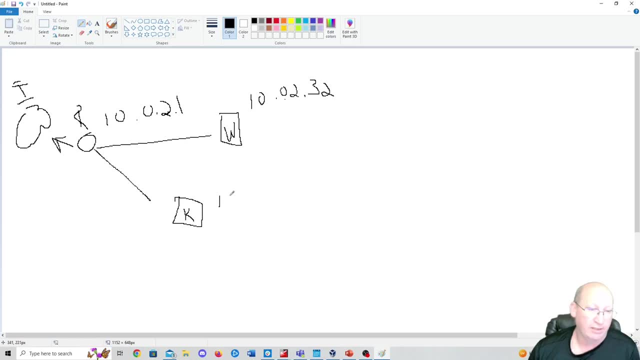 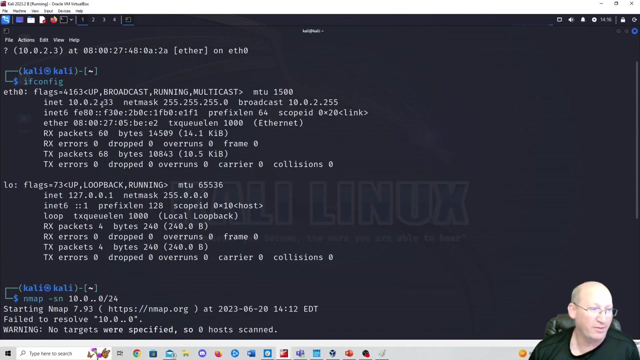 and then our cali box right here. that's on 10.0.2.. what do we have? is that 133? i'm really bad at addresses. what can i say? i'm? i need to work on it. that's a big deal. uh, so that one is on 33, so it is on 33, okay. 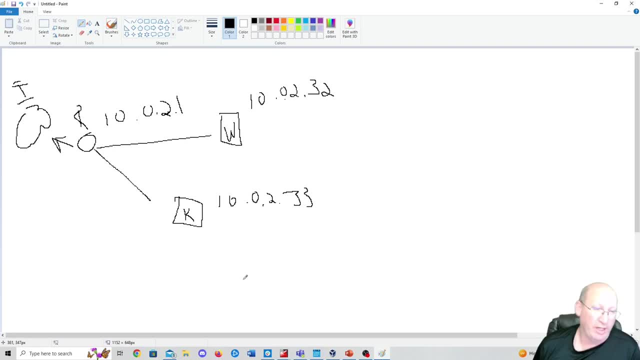 so we're on 33, right here now. what we're going to do in a current, in a normal network? right, we have an intrinsic trust system. so the windows machine is going through the router to get to the internet and our cali box is going through the router to get the internet. what we want to? 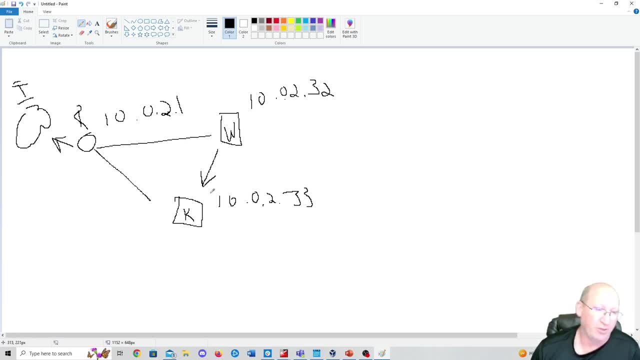 happen is we want the windows machine to go through our cali box to get to the internet, which will allow us our cali box to kind of do a man in the middle attack and allow us to do some other weird and freaky things. uh, and that's where art poisoning comes in. the reason it won't 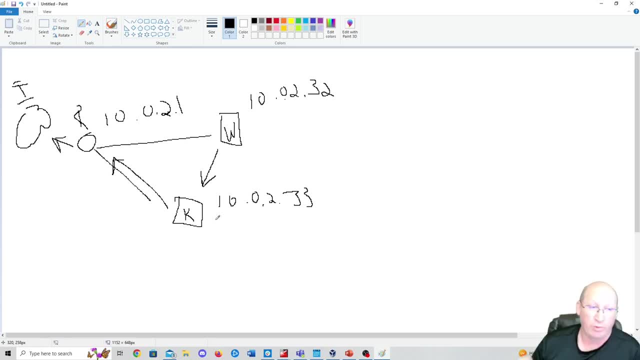 work in my virtual environment, in my normal home lab setup, where we're using the firewall, we're using all those other things, is because this windows box is usually set up as a static ip and with a static ip it knows that the default gateway is 10.0.2.1, it knows the mac address, it's. 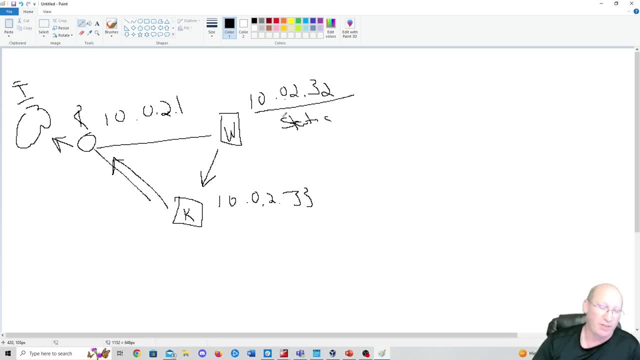 not going to change it right, so that's kind of the the way to get out of this. but if you're ever at, like a starbucks, an open wi-fi system, something like that, you'll hear us in cyber security constantly tell you: do not get on open wi-fi systems. and this is one of the reasons why. 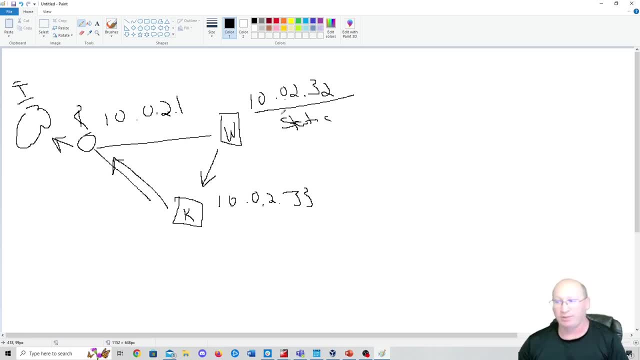 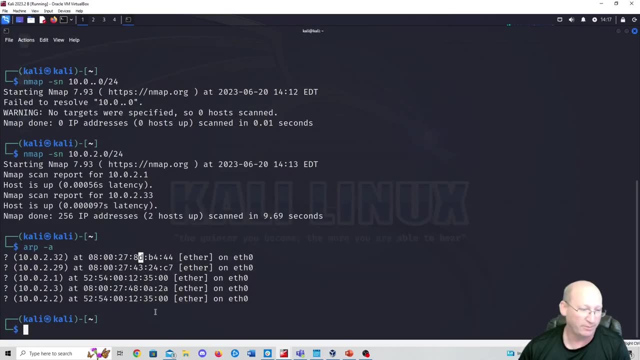 there's other reasons as well. right, i could do a rogue access point, uh, which kind of does something similar, but this art poisoning attack is just one of many attacks that we can do. so let's jump into this, let's kind of go through it a little bit. we're going to use a program called better cap. 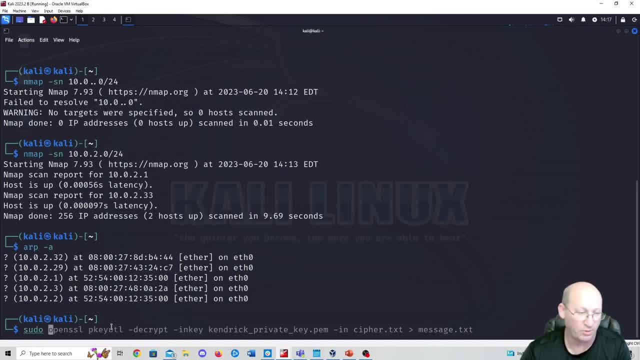 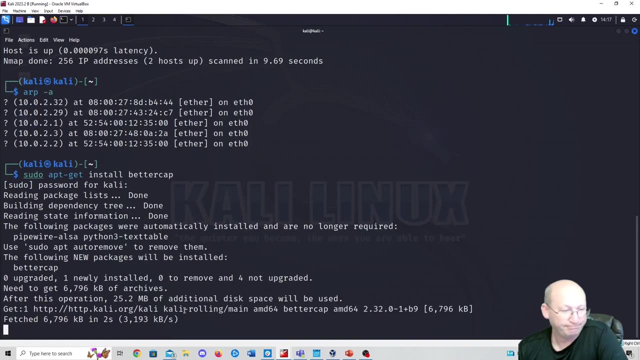 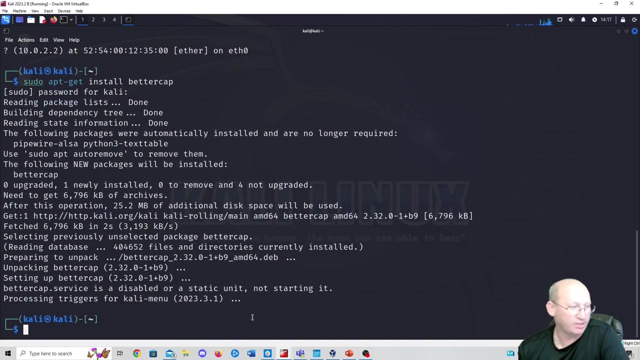 and the first thing we need to do is install it. so i'm going to do a sudo apt dash get. install better cap b-e-t-t-e-r-c-a-p. we're going to install. that shouldn't take too long, okay, so that one's installed. 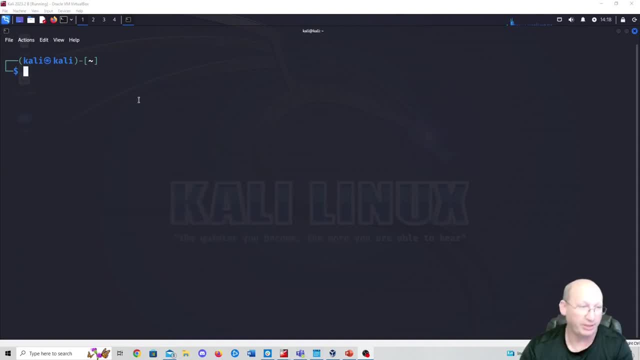 so in order to initialize it, we're just going to type in better cap, like so, and you'll see that it's giving permission to deny. we need to be in root, so i'm going to go ahead and go up to the very top. i'm going to click on this root terminal emulator type in that trusty 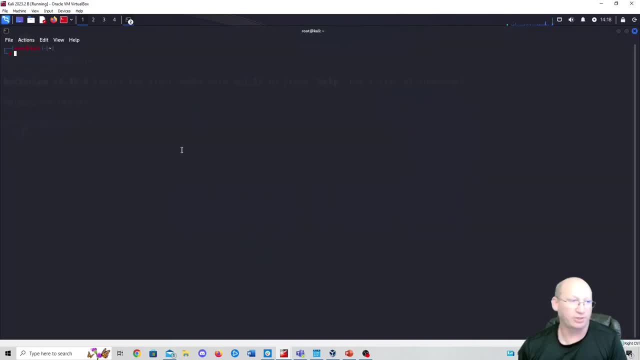 password. it's going to give me access to the root terminal and blow this up a little bit for you. and now, if i do that, i'm going to be able to install better cap b-e-t-t-e-r-c-a-p type in better cap. i shouldn't get permission denied, and you can see here that it's providing me. 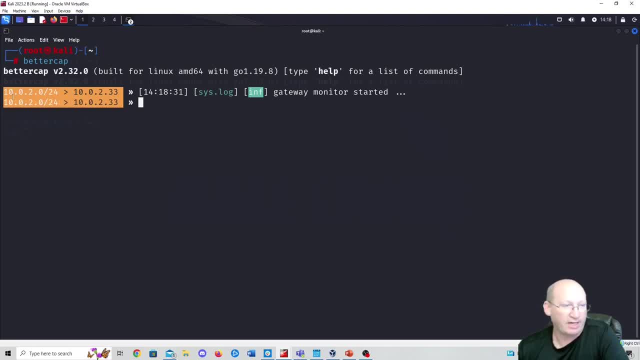 our current ip addresses, right? it's saying: hey, we're on the 10.0.2 network with a slash 24. that's at like last cider, which is going to be 0 to 255, so 10.0.2.0 through 255, and we're currently on 2.33. 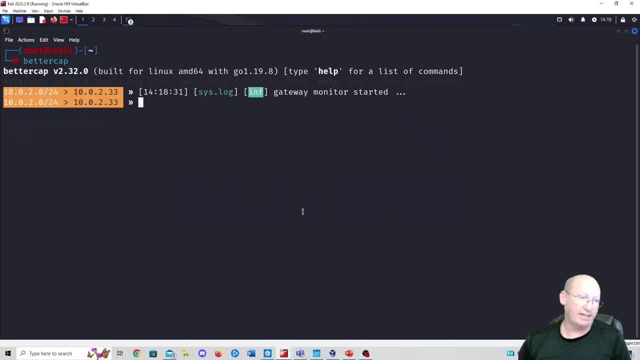 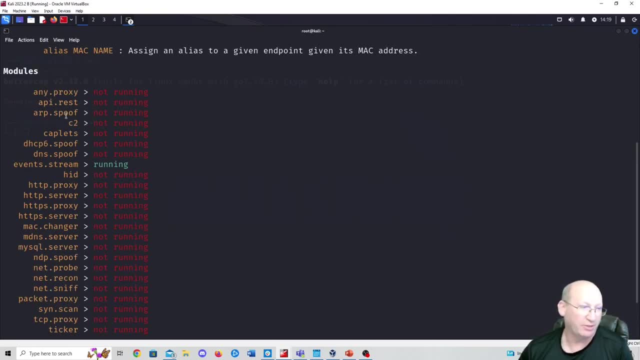 for our current system, like any other normal linux system. if i type in help, you'll see that it's providing me this, uh, this kind of information here. right, it's telling me: hey, the proxy isn't on, it's not running, arp spoof isn't on, c2, our caplets, so on and so forth- the only thing that's really running, right. 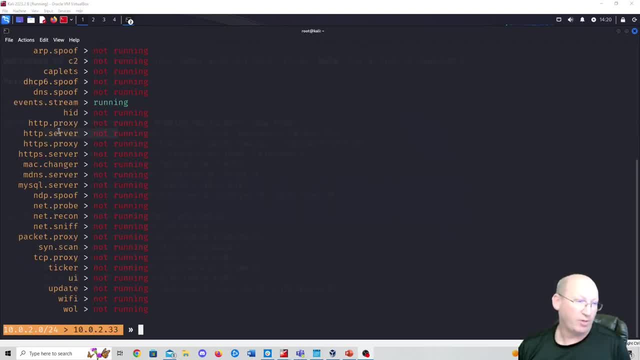 now is our eventsstream, which is fine. now, if i wanted to know about any of these, let's say that i wanted to know more about, uh, wi-fi, i could do help. and then type wi-fi. it's going to provide me kind of a associated commands associated with it. it's going to tell me how to do all this fun. 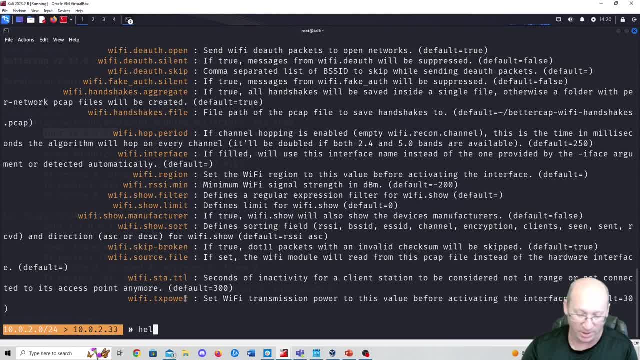 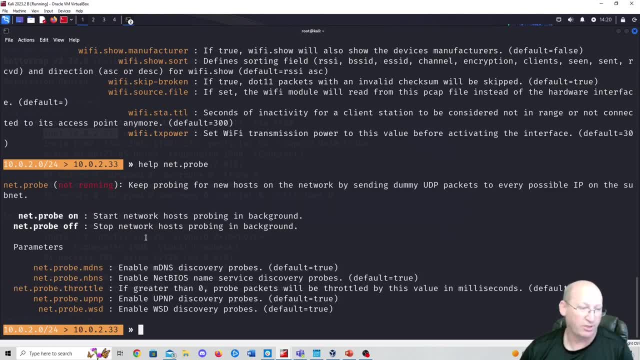 stuff. uh, in this case we're going to do helpnet probe, so help netprobe. and if i see over here you say net probe's not running and i could turn it on or i could turn it off, depending on what's going on. in this case i'm going to type in netprobe and then 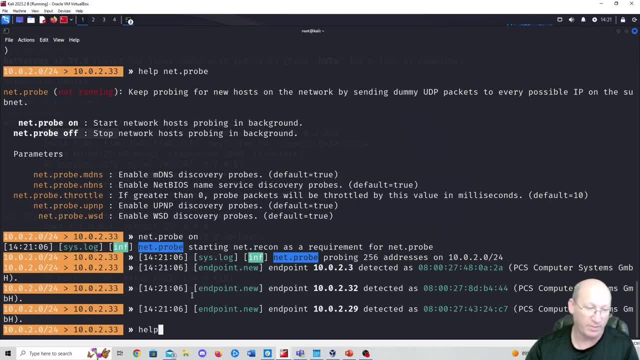 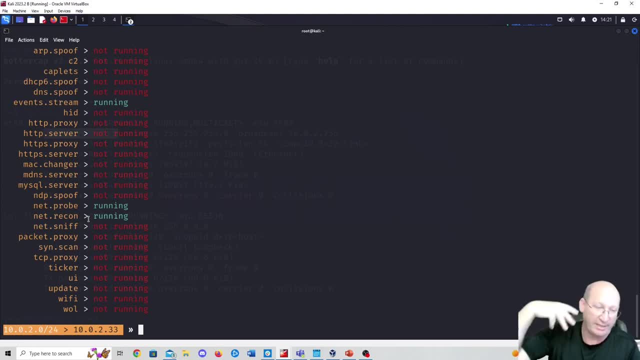 i'm going to type in on just like so, and if i type in help again, you'll see that now net probe and net recon are running. now, recon is going to basically track and and look for devices and other computers that are currently on the system, and the probe is searching for those little devices. so it's they. 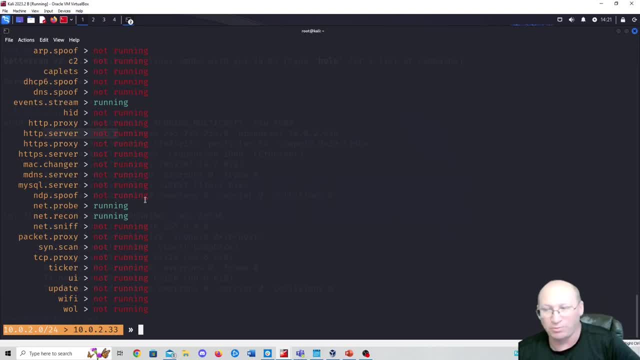 have a lot of the same thing. uh, net probe is more about probing the, the ip addresses on the same network, where net recon is more about grabbing those. if i was attached to several different networks at the same time. right, so they are attached. they're very, very similar in the aspect. 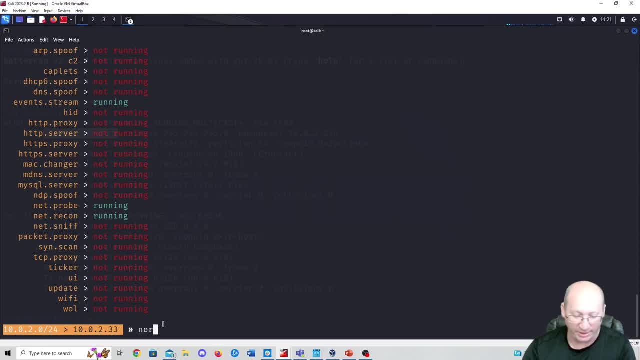 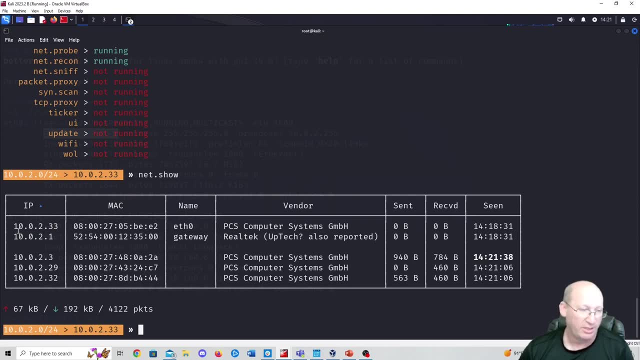 of it. okay. next one we're going to do is a netshow. if i do a net show, it's going to show me all the current devices on my network. you can see here that i got 10.33. this is the computer that I'm. 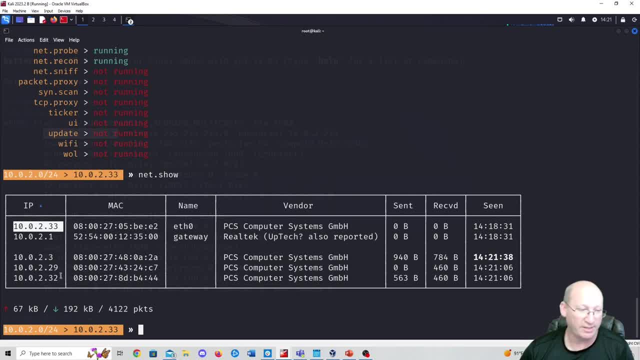 using 10.1, that's our gateway. 2.3 and all these other devices. uh, it's just kind of throwing us out there and saying, hey, how much information has been sent, how much has been received, and when we last saw these devices. so obviously we know that 2.29 is our current firewall, which we're. 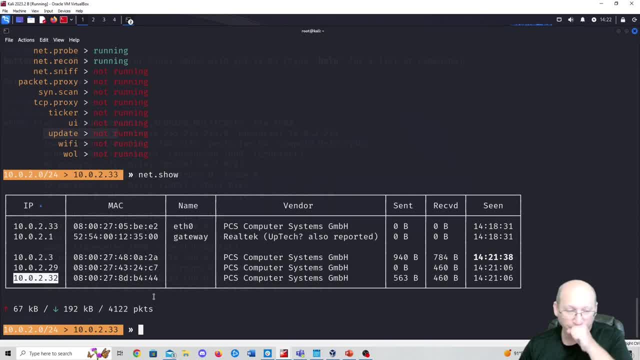 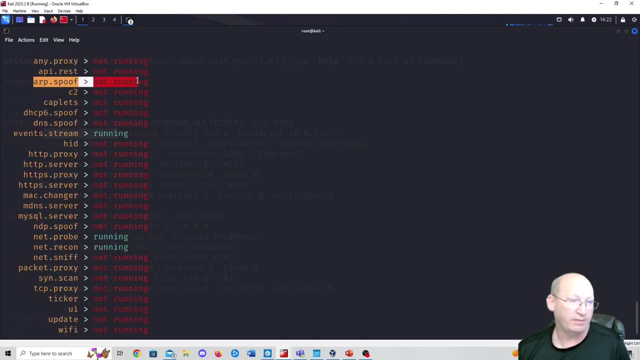 not really worried about, and 10.2.32 is our Windows system that we have on the same network. so we want to uh kind of start a spoof, right? so if we type in help again and if we scroll up we can see this ARP spoof right here and it's not running. so we're going. 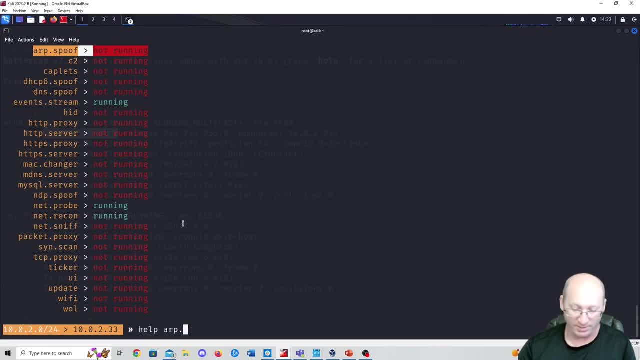 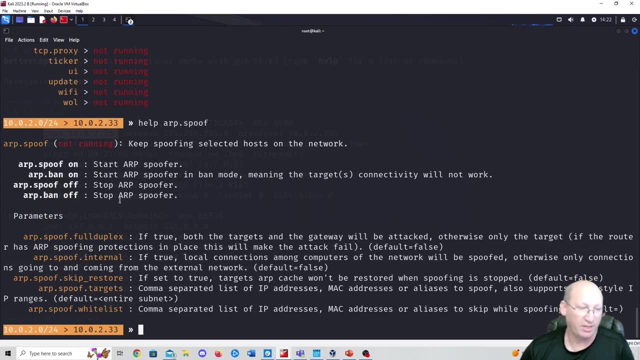 to do a help: ARP dot spoof, and we can see here that we can do ARP spoof on, we can do an ARP ban. we turn it off and we turn the ban off. so what we really need to begin is just doing um specific commands, right? so if we look at the parameters, we can see ARP, dot spoof, dot full duplex. if true, both. the targets and the gateway will be attacked, which means I'm hitting both the default Gateway, but I'm also hitting the Windows machine at the same time, and that's really what we want to do. so we're going to do: set ARP, dot, spoof dot, full duplex, and you. 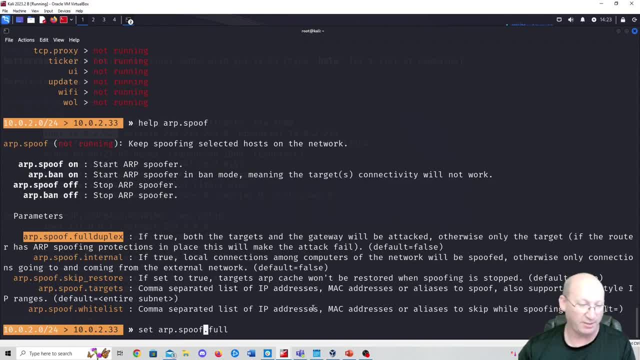 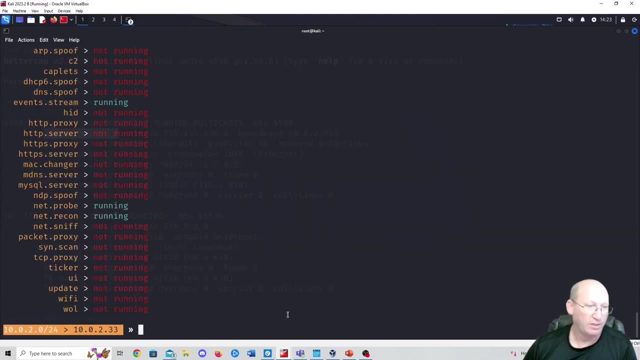 can see that right there, that full duplex and no spaces- I don't know why the spaces full duplex. and then we're going to type in true because it tells us, if true, we see on over here, we see true and we're going to doãy. so I'm going to do it right here, I'm going to save 민주 that one. 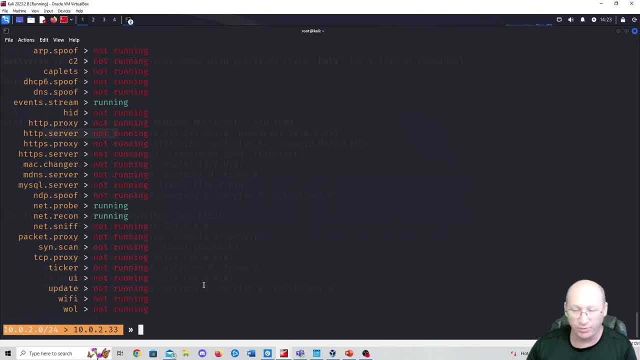 okay, so lemme re-중에 it. okay, so I'm going to set ARP dot spoof dot target this one and I'm going to run this command and the command C seguirlist. let's move this command. okay, and we're going to do help'. OK, so we're gonna turn that on and if we do help again, you can see that ARP spoof is still. 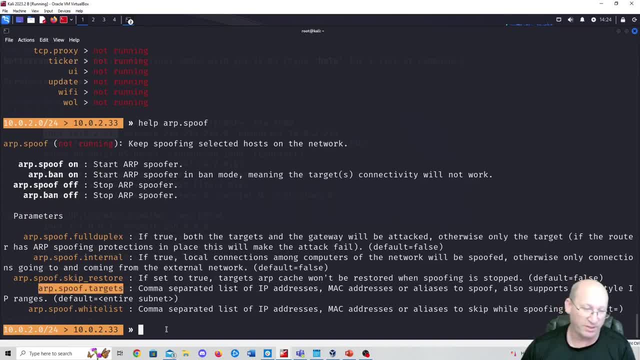 tells us arpspoof targets, comma separated for list ip addresses. so very easy tool. so i'm going to do cell sets- excuse me, arpspoof dot targets, and i have to define what i want to attack. well, i want to hit the router, so that's 10.0.2.1, and then it says right here: uh, put a list of ip. 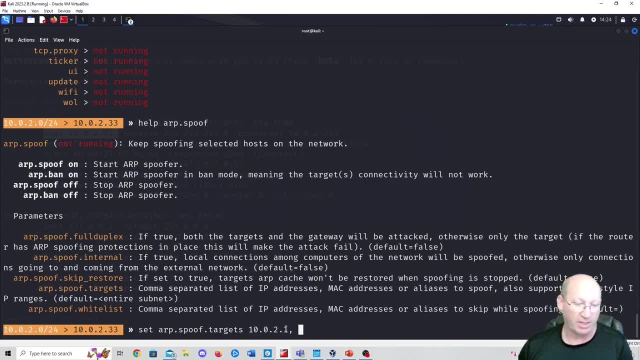 addresses, mac aliases, so on and so forth, uh, separated by a comma. so we're going to hit both ways. since we're on full duplex, we can hit both the router and the windows machine, and then we're going to do 10.0.2.3.1, i believe was what our windows was at. let me double check on that one. 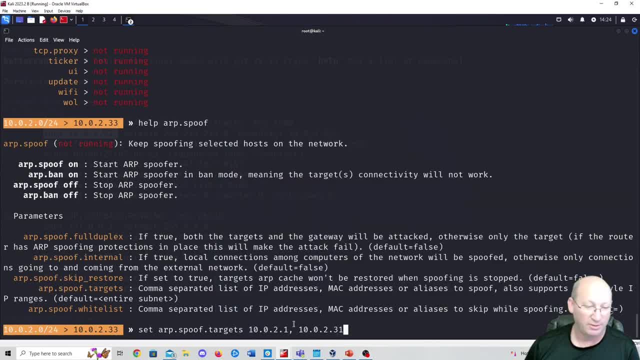 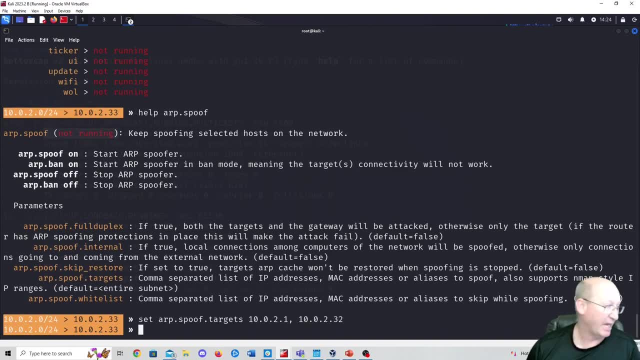 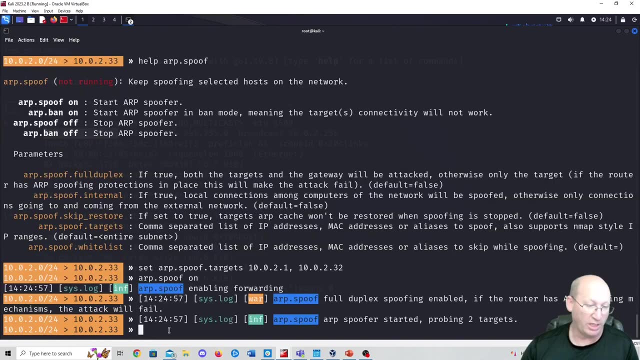 and we can see here, our windows is at 32, so let me change that to 32 and then we'll set that, and now we're ready to actually perform the, the attack against the target. okay, so we're going to start real quick, we're going to do arpspoof and then, on, this turns it on and if i do a help. 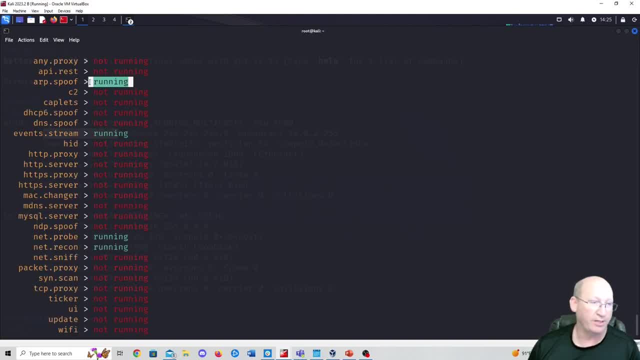 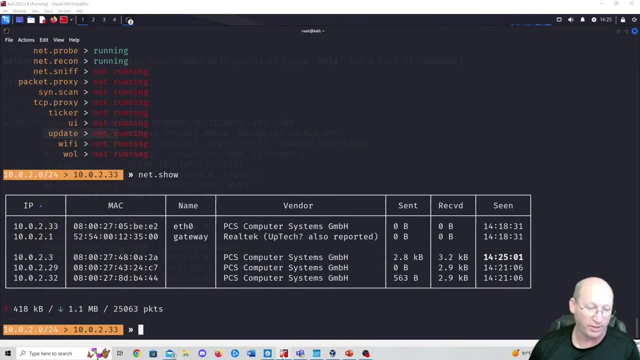 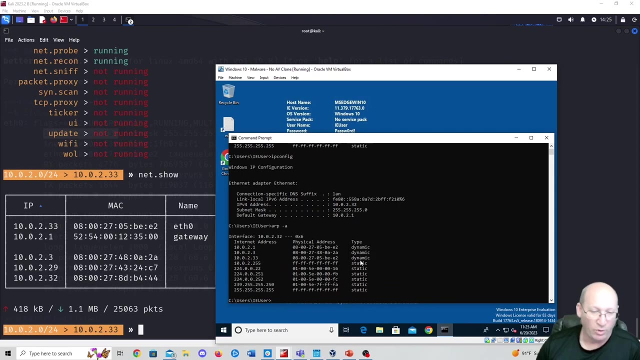 we can see now that we're running that arp spoof right there. okay, so i'm going to do a netshow. let's go back into our windows system and see what's going on over there. so if i go back into windows and we do an arp dash, a right here, i want you to see what's. 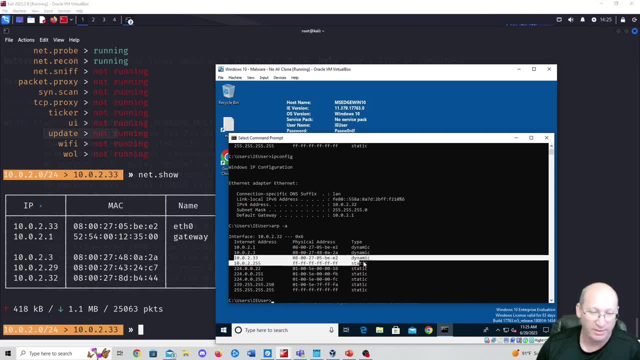 going on here. right, here's our 10.0.2.3.3. right we can see the mac address 08002705be-02, and now you can see the gateway also has that same mac address. so we have successfully spoofed the target machine with the router. and if i were to plug into the router, if this was a normal router, 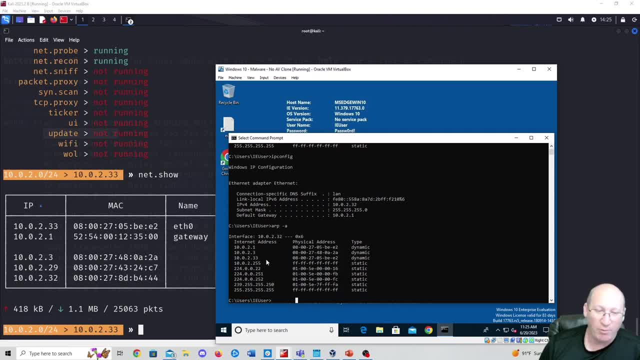 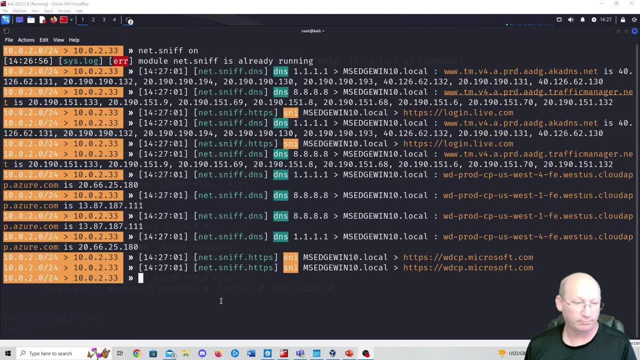 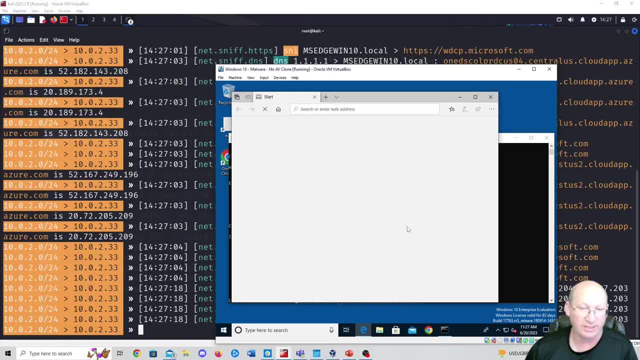 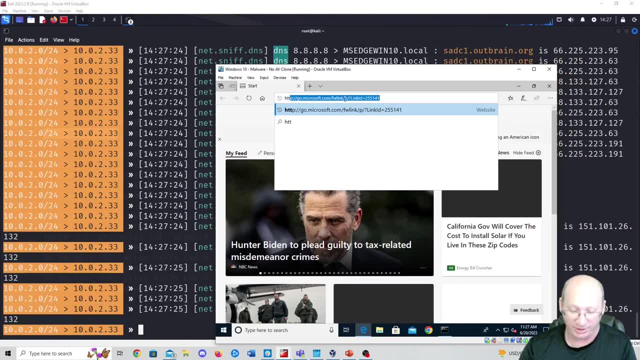 here. let's go on to. i'm going to use- uh, i used google last time, i need microsoft edge. this time we're going to just go to a plain text website, not something that's not https, right? so we're going to do http colon: forward slash, forward slash. i'm going to do unicorn items, unicorn. 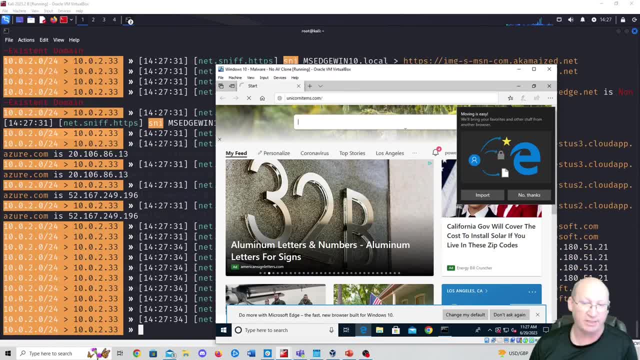 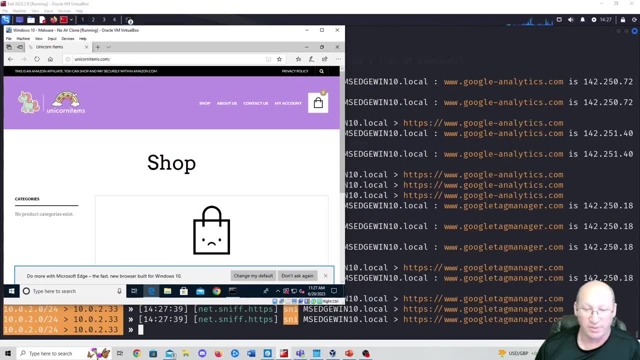 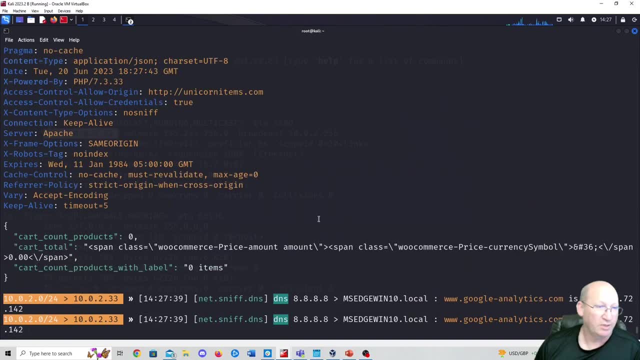 itemscom. this is an http site and no thanks. and let's kind of see what's going on over here. right, i've got unicorn items and you can see that we're doing google manager. we could see all this good little analytics, okay, but let's see. 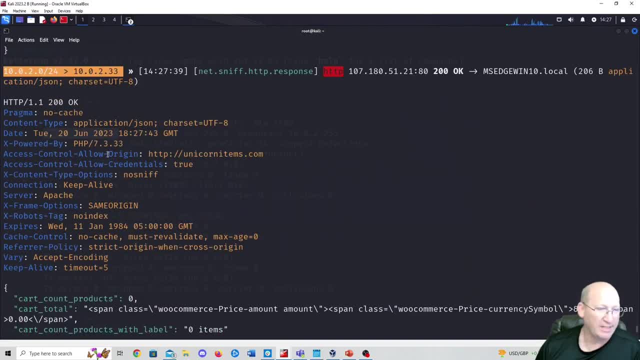 what's going on up here? if I come up a little bit, I can see that my Cali box detected my Windows machine access in the site unicorn items- calm, we can see that as access control. let's log in. let's go back into that Windows machine. 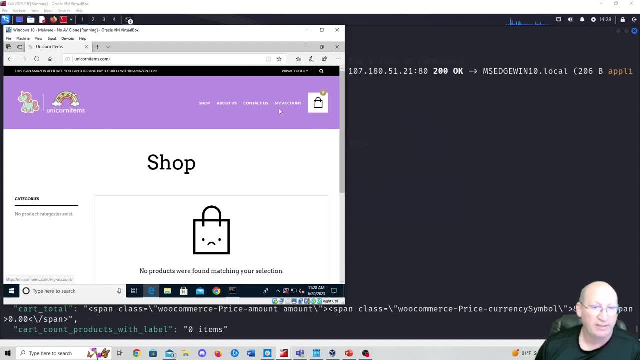 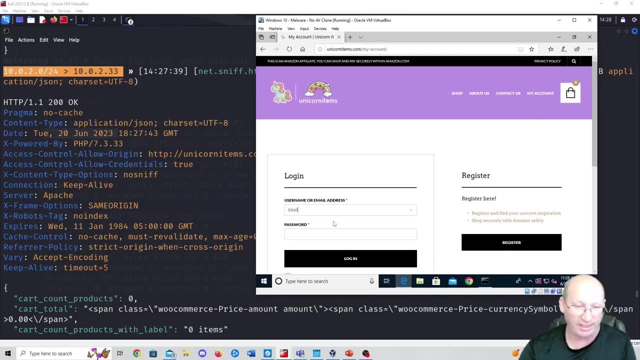 and I'm gonna say: don't ask again and let's do my account. now I don't have an account with them, it's not a big deal, all right, but let's just type in something I'm gonna do: chat at hotmailcom, and then I'm just gonna do a. 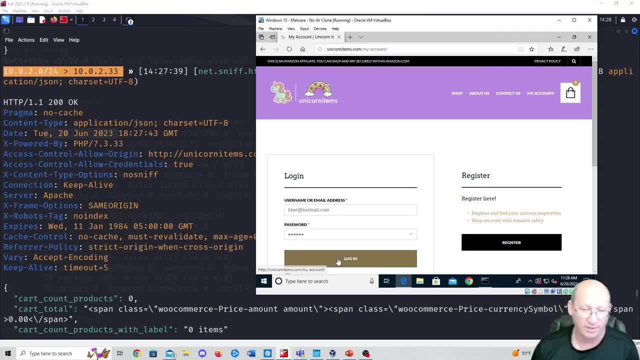 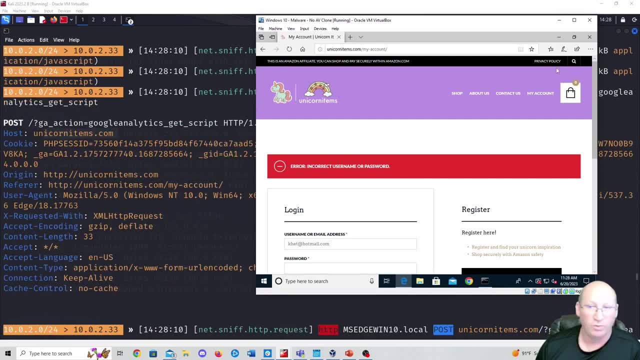 password: 1, 2, 3, 4, 5, 6, and I'm gonna log in. I'm not gonna save it. well, I guess I did save it. let's scroll down a little bit and see what's going on now with this. alright, so this is where we try to access the site. I can see unicorn items. 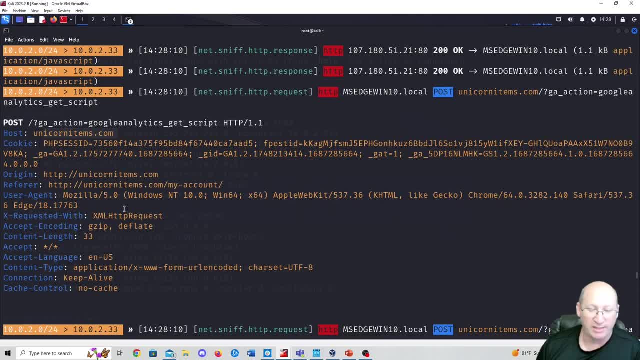 calm, we can see the account now. this is because it's going through the Cali box to get to the internet. you can start to see the information that's being passed down. right, we can see the refer agent. I should be able to see the actual script. 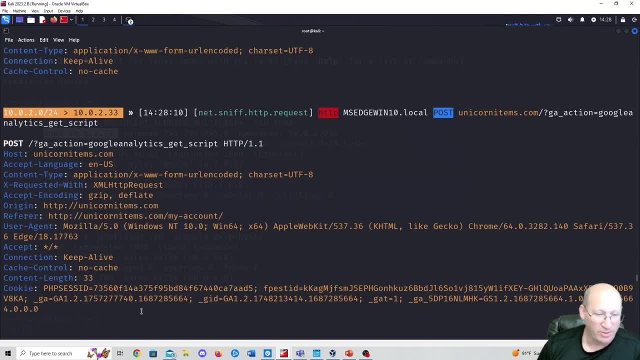 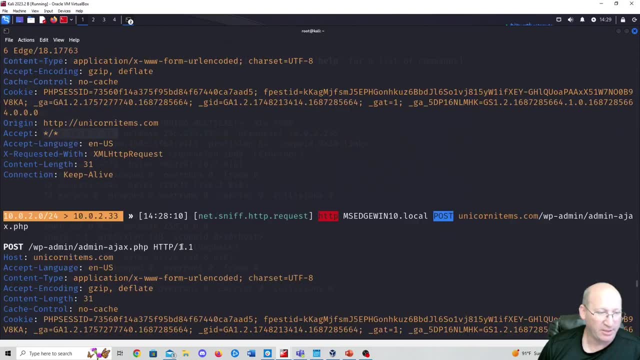 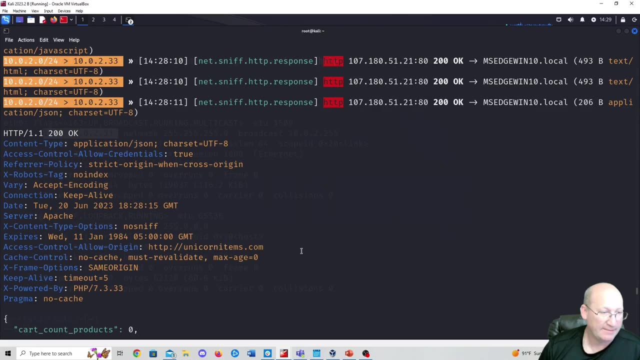 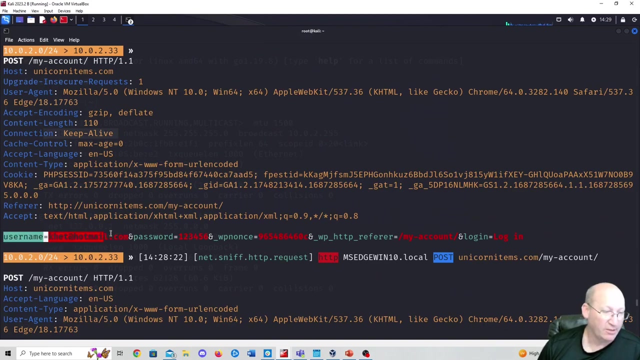 in which case we tried to log into the website. so we see the cookie here which we could utilize an attack later on the road. let's see what else do we got here. keep alive, keep alive. here we go. I'm doing the right way, K farewell, like a thing about actually moving from. oh, you can see right here a little bit. 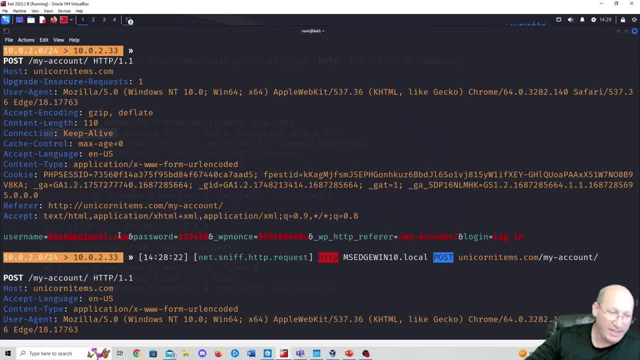 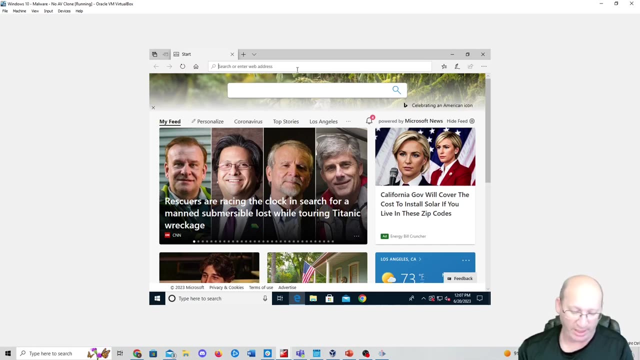 ways down the road that the user typed into this website, chatted hotmailcom, with the password of one, two, three, four, five, six, and it's printed out there in red. because we're conducting a man-in-the-middle attack, because the actually do a little bit different, right, we're gonna do a, I don't know, let's do. 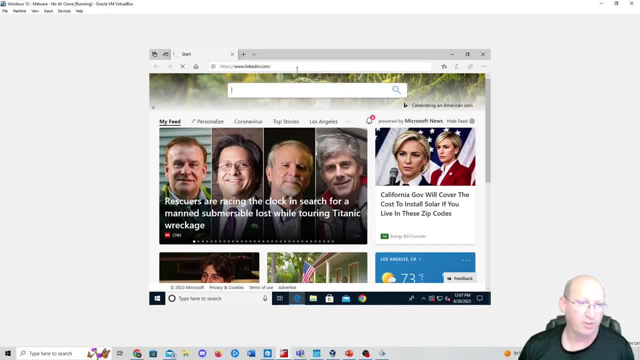 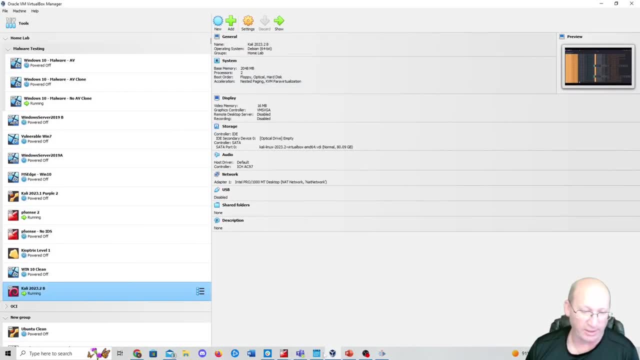 let's do LinkedIn. so LinkedIn calm. now. LinkedIn is running HTTPS here. I'm gonna go ahead and try a sign in. let's go back to our Windows box over here, or, excuse me, our Cali real quick, right, but it's not really detecting that we hit. 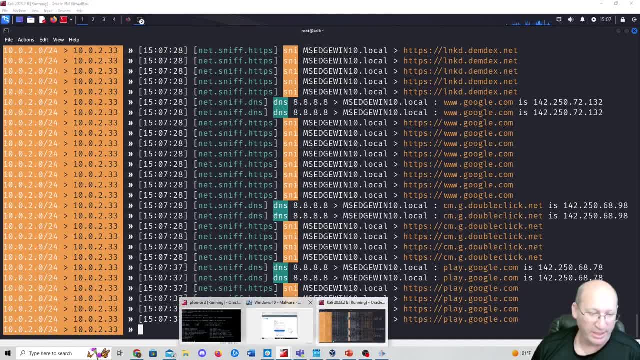 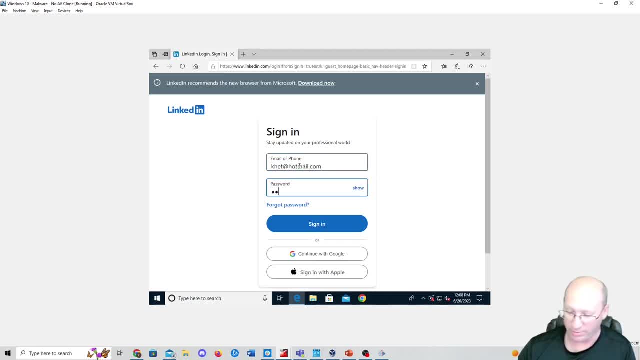 LinkedIn like it did before. right, and that's because we're on an HTTPS site, so let's try and hit there. so I'm gonna do chat at hotmailcom and again we'll do that password of one, two, three, four, five, six. we're going to hit that sign in. 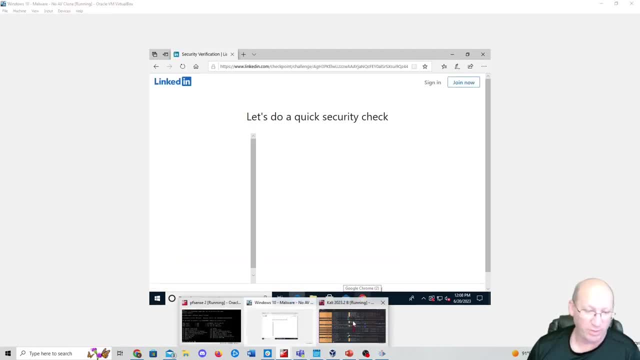 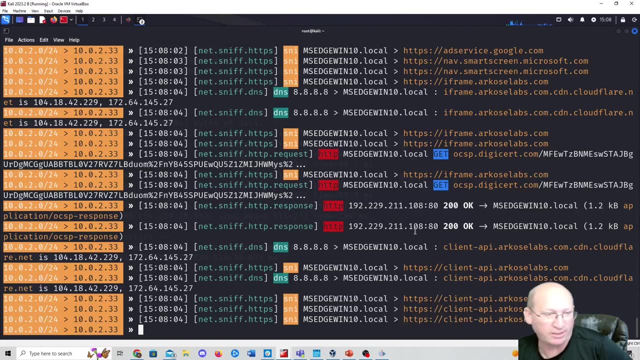 I'm gonna hit never it's gonna try and detect it. let's go back into our system here and you can kind of see that it's not giving us near as much information as it did when we went to an uncalculated site. right, we can see Bing. 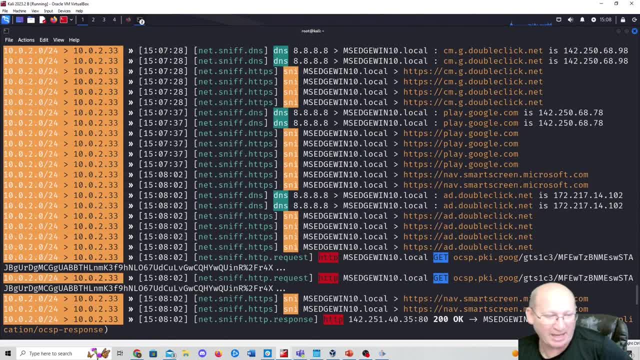 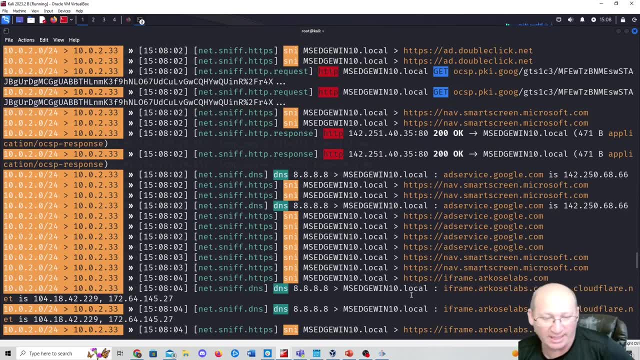 but we're not seeing LinkedIn hit in at all. we're not seeing the username, we're not seeing the password because it's all encrypted. it's all using that, that transport layer security, that SSL, to hide that information from us. okay, we can see that it's hitting this DNS, right? 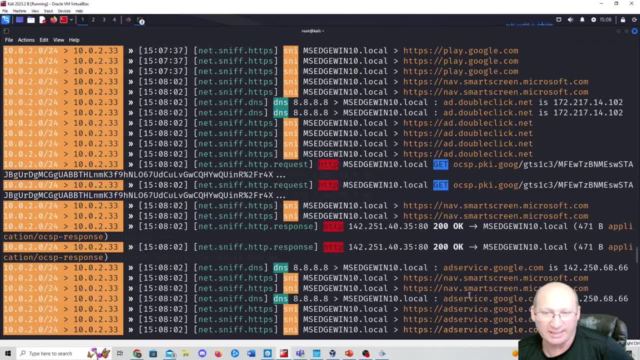 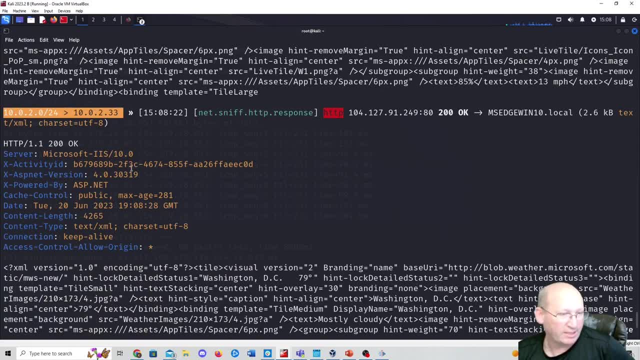 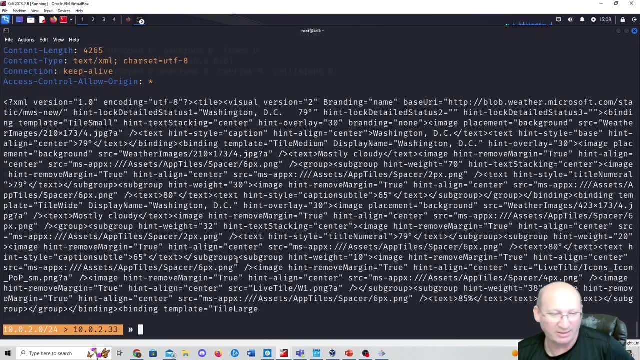 but again it's not telling us where we're going. it's not telling us anything pertinent because we're doing HTTPS right? if I scroll down a little bit more, we can see here it's saying activated. before it showed us that we're going to unicornitiscom. now it's not telling us anything. it's literally. 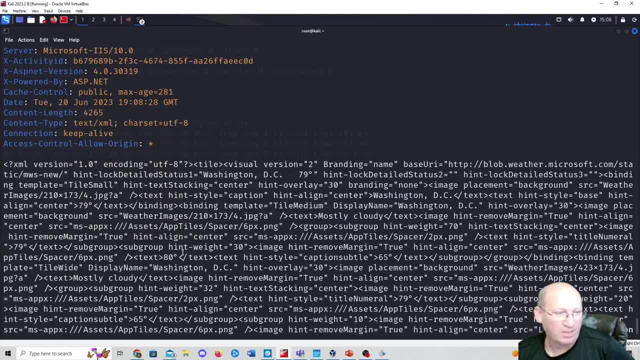 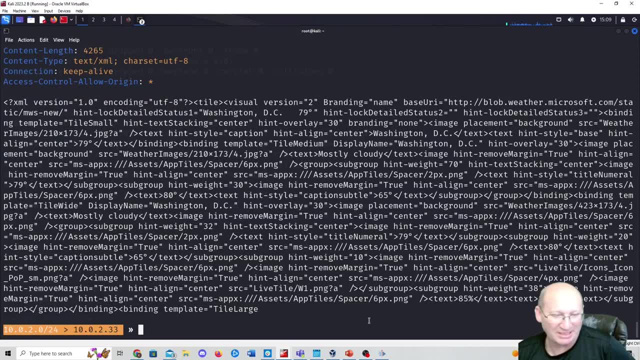 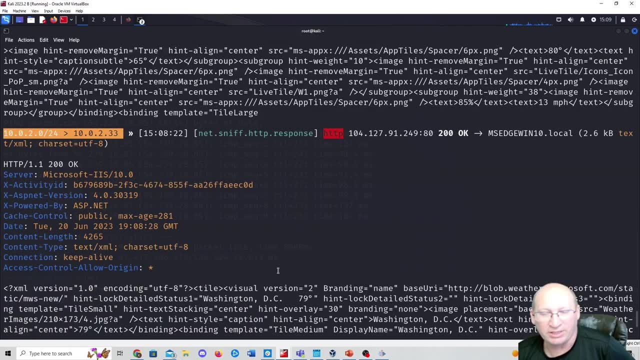 pretty much blank in every aspect. right, let's see here. it's not telling us the name, it's giving us the weather for Microsoft, it's just. it's just not giving us anything. we just don't have anything, like we did before. so the object at this point would be to get the attacker to, not to, downgrade. 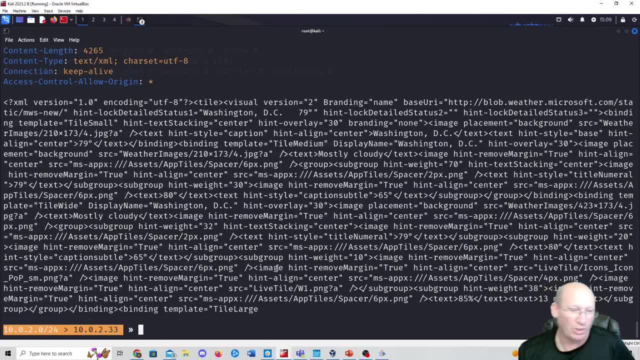 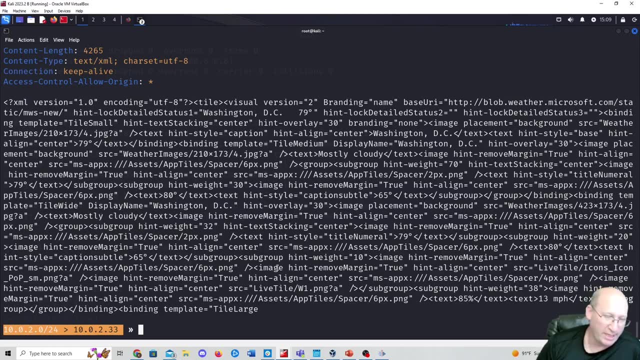 their attack. right, if I was in a malicious actor, I would want to take that LinkedIn, that HTTPS LinkedIn account and I would want to downgrade it down to HTTP. however, a lot over the last decade websites have been removing that. there used to be about a decade ago where you could take an HTTPS website and 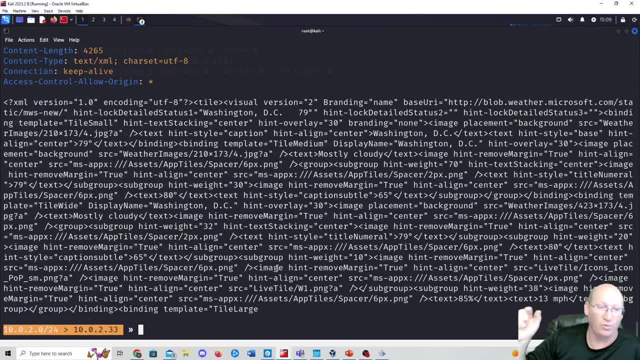 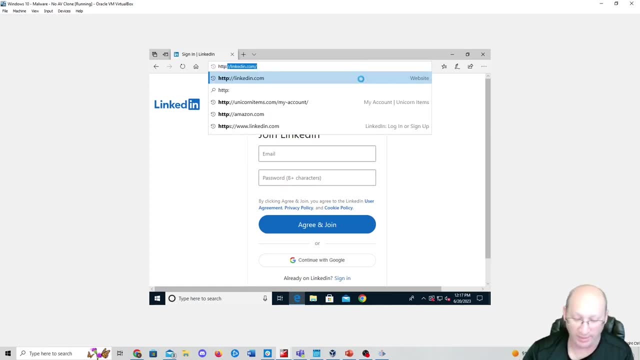 they had both an HTTPS and an HTTP and if you're well, your browser didn't support HTTPS, then it provided that HTTPA as well, and as I'm down on the middle attack, you could do a downgrade attack. so let's see what happens here when we try to do that. right, if I want to do HTTP- I left off the ass, I can do. 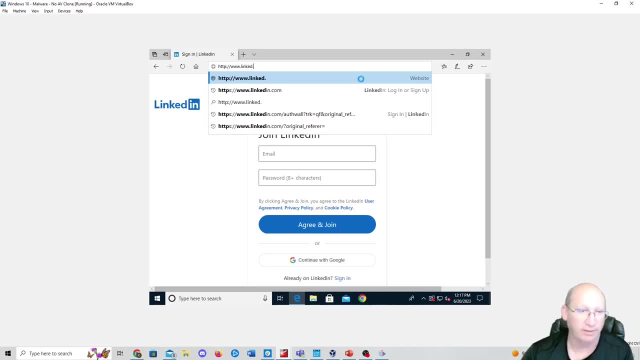 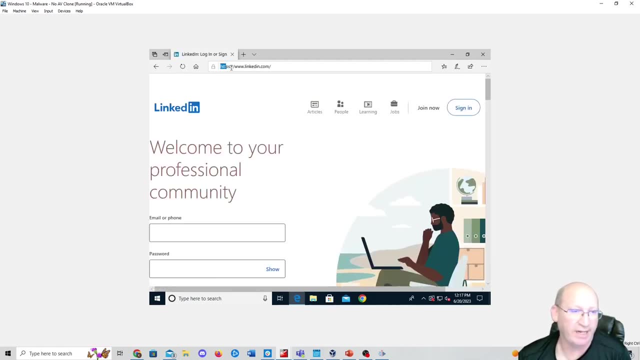 forward, slash, forward slash. wwwlinkedin, LinkedIn, incom, and you can see here that it's going to kick it back over and it made it HTTPS, and so a lot of those vendors, a lot of those websites now don't allow you to do a downgrade attack at all, so it's almost it's an old-style attack, not really. 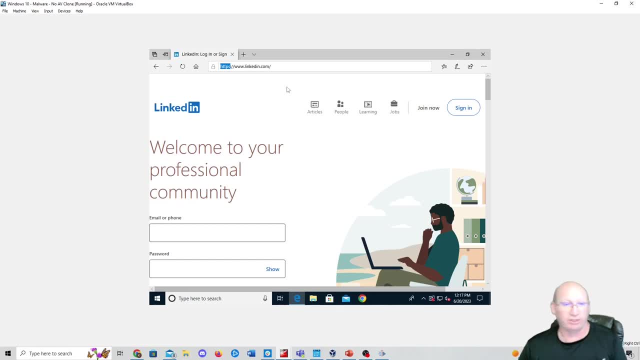 prevalent today, and so my other option, if I was a malicious attacker, would be to clone this website and then do a DNS spoof and then force that traffic that would be going to LinkedIn to go on to my LinkedIn page on my web server, and that's where this type of attack is a little bit more advanced. it requires a 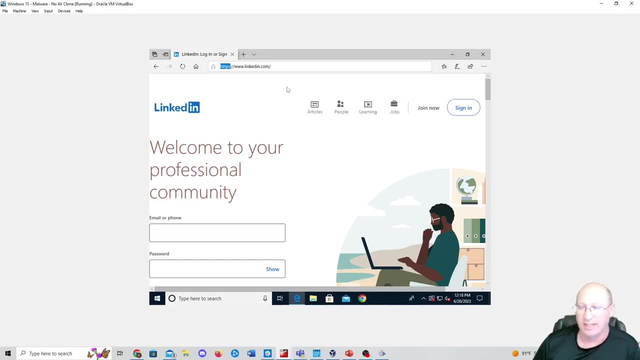 little bit more to do, but you would have to be logged in as well as to do it, and that way you could force the user to thinking as long as they didn't see that lock sign at the top or that HTTPS, you could technically fool the user into. 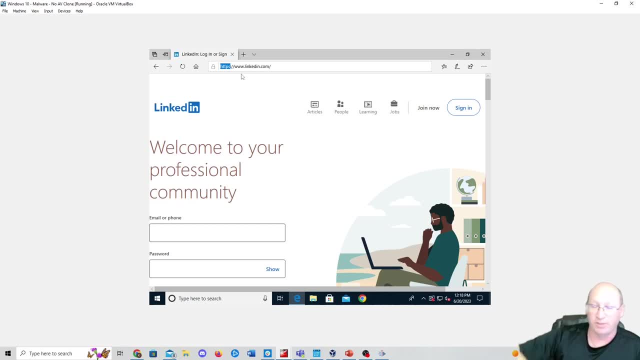 thinking they were really logging into LinkedIn, and then, of course, once they logged in, you just forward that, that information, over to the legitimate website, and so they don't know anything's going wrong and we're seeing that type of attack still for man in the middle, but a little bit more complicated than 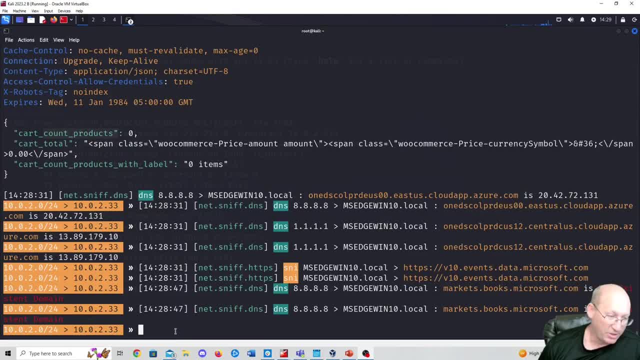 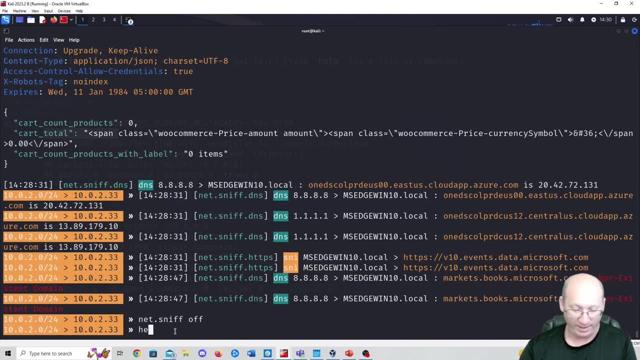 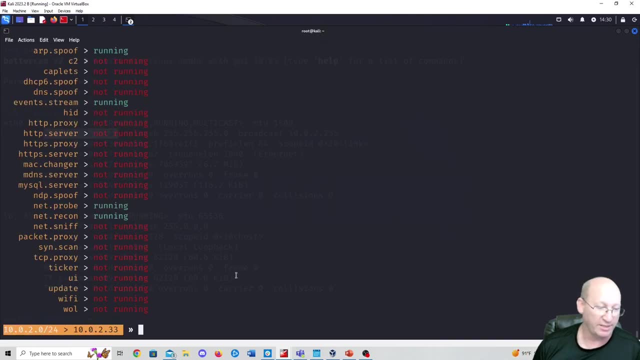 what it used to. be all right, so I'm going to turn this off. we're gonna do net dot sniff off. I'm gonna do a help just to see what's going on. still, we can see net sniff is no longer running. we still have access to the art table. we still have access to. 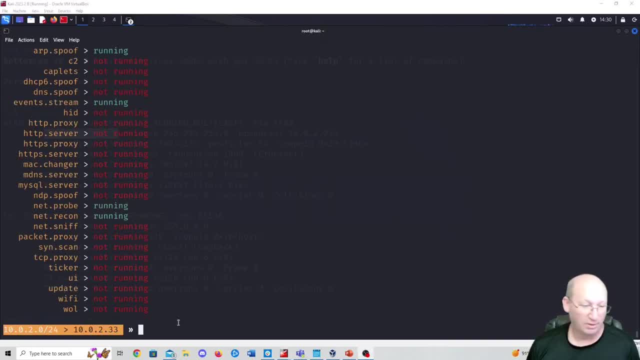 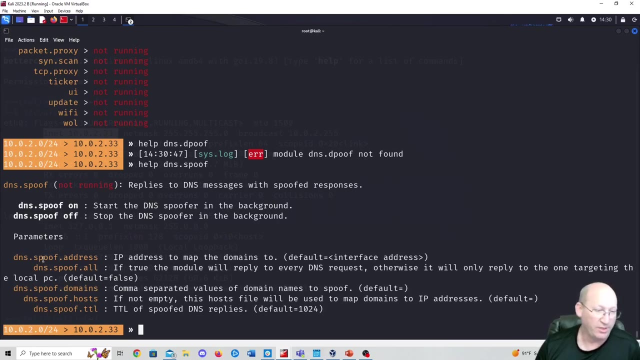 that machine, but let's see if we can't do a little bit more. so, just like before, we're gonna type in help DNS dot spoof. if I can type today, which I probably can't spoof, we can see here that it's not running. to turn it on and off, we can also do a DNS. 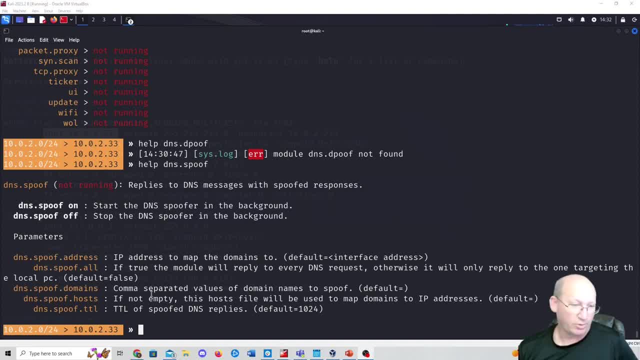 spoof address IP address to map to domains too. so we're gonna spoof a DNS right now. DNS is a domain name service that basically translates an IP address into a common name. so in computer language I'm not just going to amazoncom. what my computer needs to know is the IP address for amazoncom and if I open up, 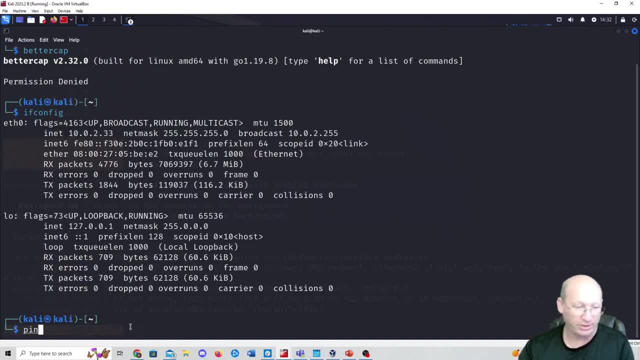 a new system right here I can actually do a ping amazoncom and it's going to actually do a ping amazoncom and it's going to do a ping, and it's going to actually do a ping amazoncom and it's going to do a ping amazoncom and it's. to tell me that one of the IP addresses associated with amazoncom is 54-239-2885. When I hit Ctrl C to stop that and what I want to do is I want to take a domain and spoof back into my id address, and so 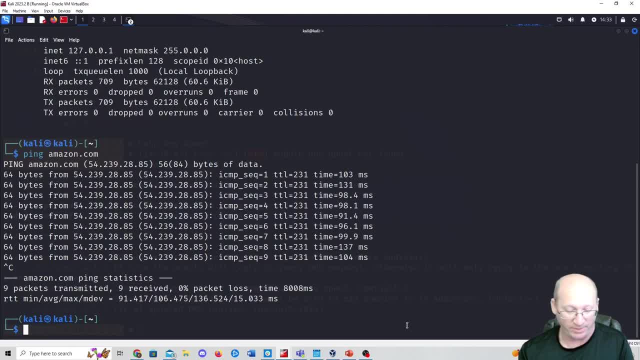 what I'm gonna actually do is I need to set up a server first off, right, so I'm gonna do Darwin serverDOM here for our bargains app. send COz, whatever server. Iranian server: Rails 2itäs start, which is going to turn. I cannot. I today is gonna turn my cali box into an. 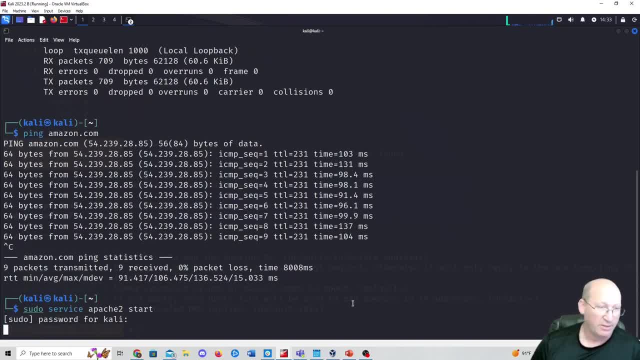 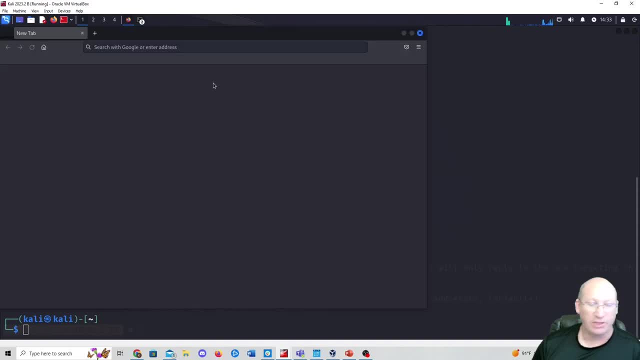 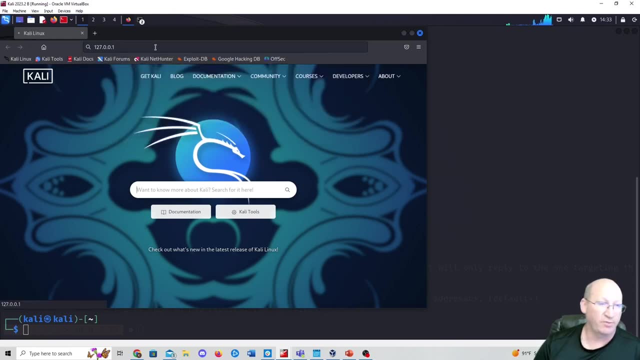 web server right. so I hit that password in there and I can prove this. if I go over to my, to my Firefox over here and I type in 127, 0.0.1, you can see here that it's gonna provide me with that. I hacked you, isn't this awesome website that we? 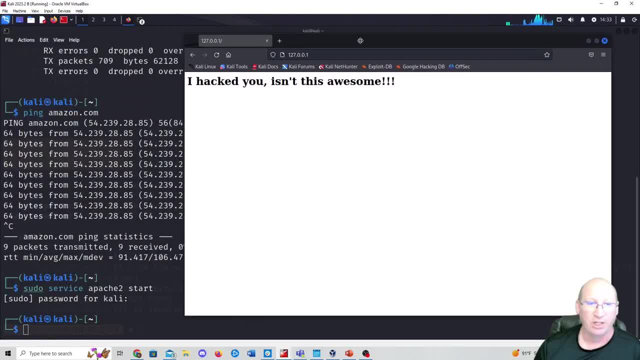 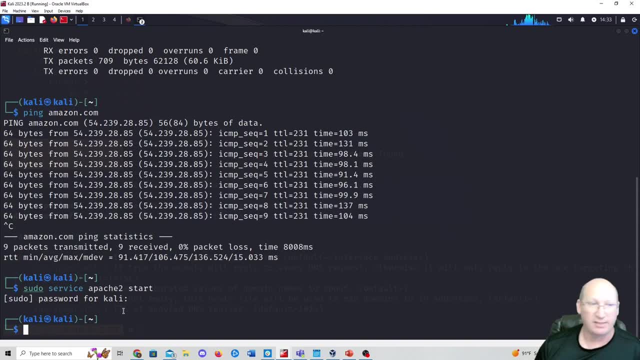 used before. right, because we set it up as index. so that's our landing page. what I want to do is I want to set the DNS to where, if somebody accesses, say, Google on this website, they're actually not going to go to Google or Amazon, they're gonna. 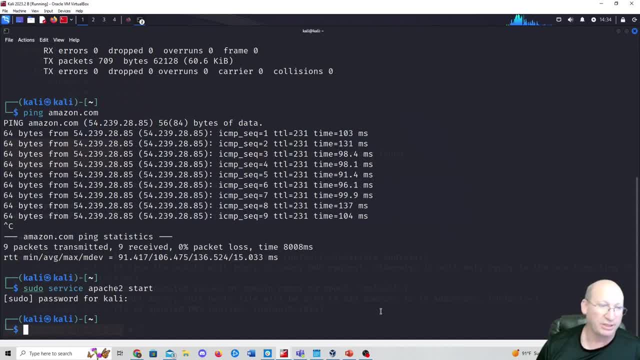 go to my website now. there's a couple conditions that have to rely on that right. this would be an incredibly insecure system. they're gonna depend upon that router for the DNS. if it's going through a specific DNS, then it's not going to work. so let's check our Windows system first. we're gonna have to. 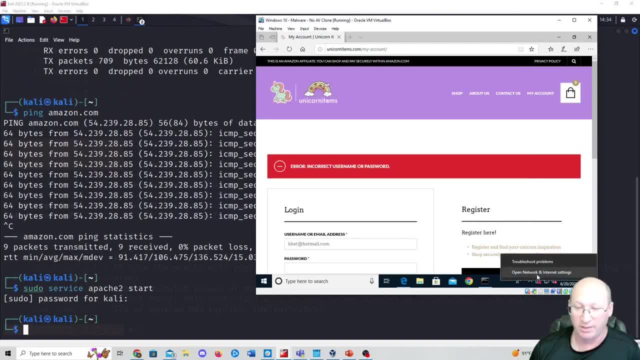 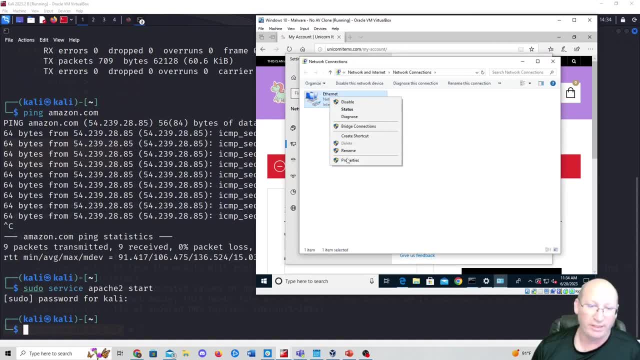 go into that command console. let me run that right click over here. we're gonna open our network settings. we're gonna check our Ethernet, change our adapter settings. I'm gonna go to Ethernet number four over here down to properties and then IV for and you can see that we have the DNS. 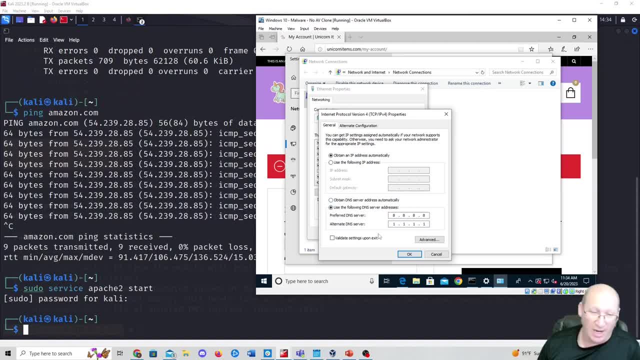 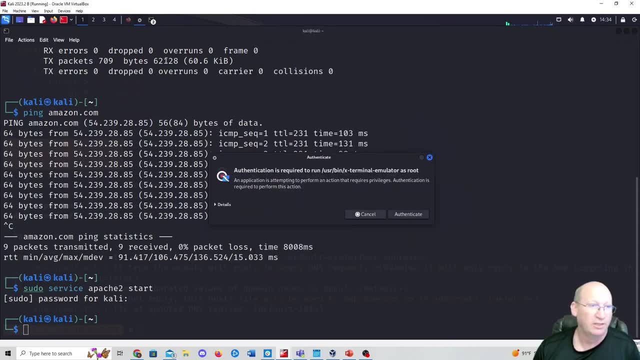 enabled right now to go to Google and through CloudFlare. I'm gonna leave it like that for right now. we're just not gonna touch it. let's see what happens, though. let's go back over here and see if this will tackle work based on this. 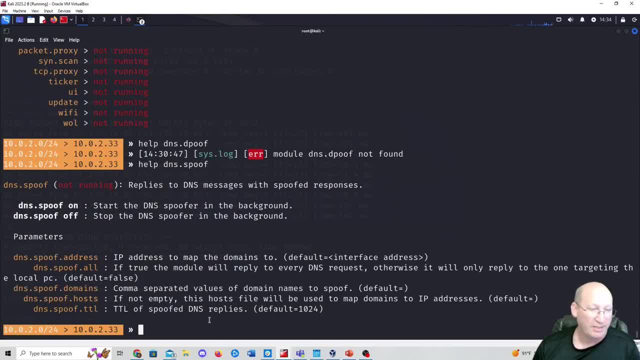 right. so let me go back over to here to route Cali. now we need to do the actual programming here to change it. so the command is going to be set: DNS, dot, spoof, dot domains, right, and we're gonna change it. let's do. let's do, amazoncom. 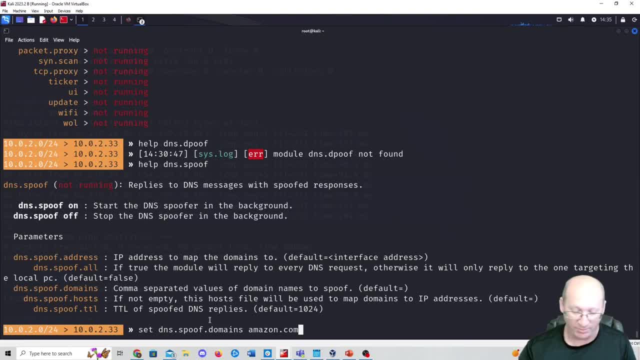 right. I mean, why not? we'll do amazoncom and then we're going to do a semicolon and then set DNS, spoof, dot address and we have to use our current address. we're going to 2, 10 dot 0, dot 2, dot 3, 3. that's gonna send the address back to. 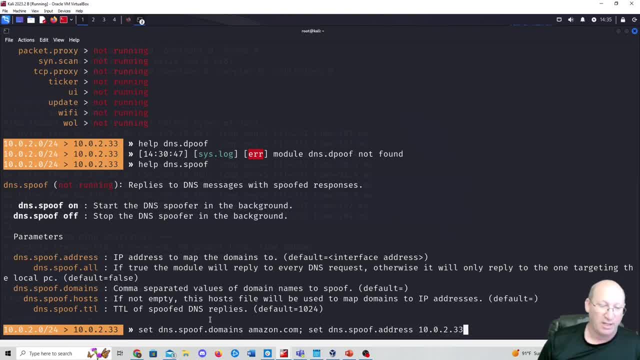 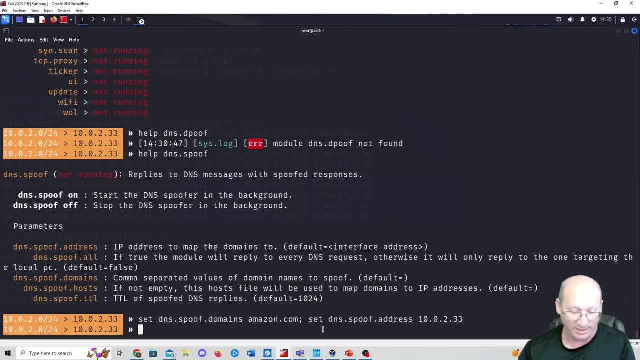 into our system right here. okay, now, this is actually two different commands. that's what that semicolon is doing right there. okay, get that. and then I'm actually gonna start the DNS. right, so I'm gonna do set DNS or not even set, sorry, DNS dot spoof, and then space on this is gonna turn the DNS spoof on. I'm 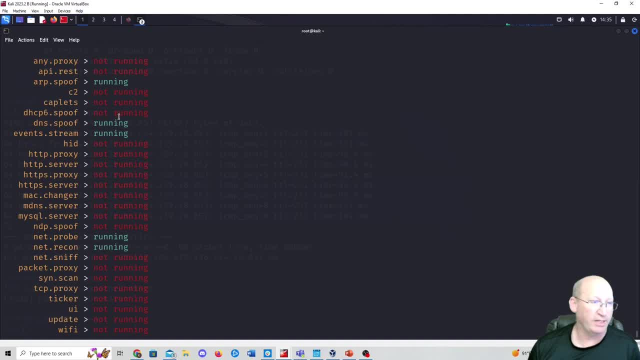 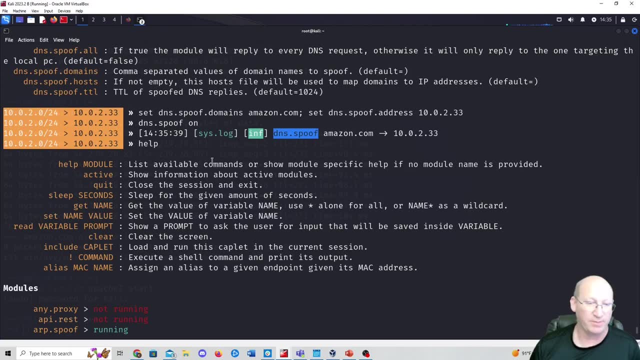 gonna type in help and you can see here that we are running a DNS spoof up here and if you look back to this command it is saying: DNS spoof. amazoncom is supposed to guard, so let's go to our Windows 10 system right here it's still. 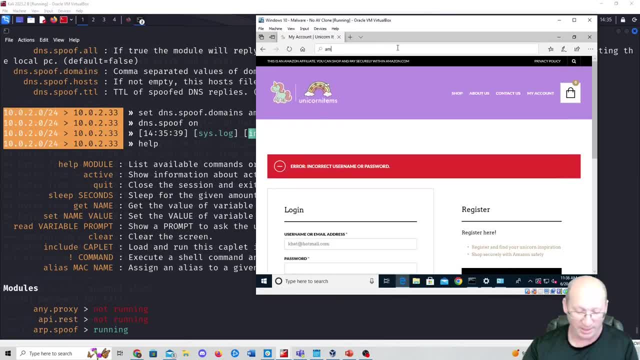 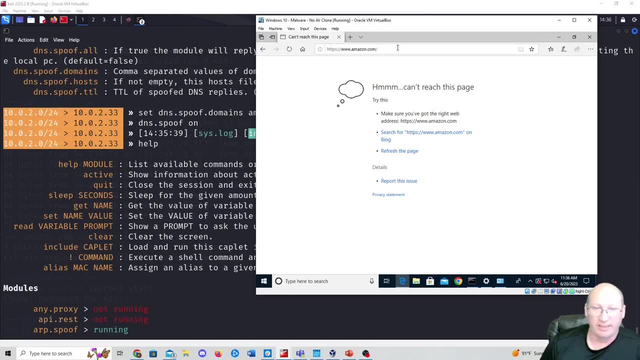 using the DNS for this. all right, I'm just gonna type in amazoncom and let's see what happens. okay, so there seems to be an issue. it's not able to click it, it's having a contradiction of terms. it's having some issues, right, so let's. 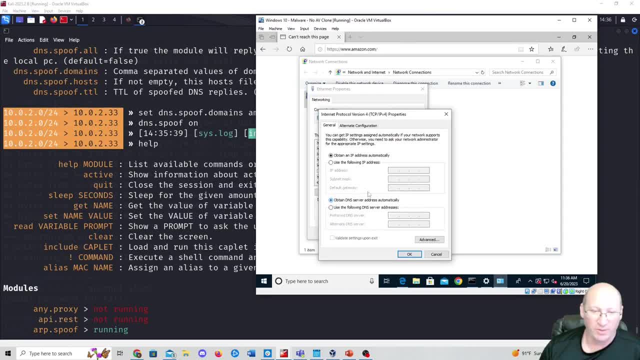 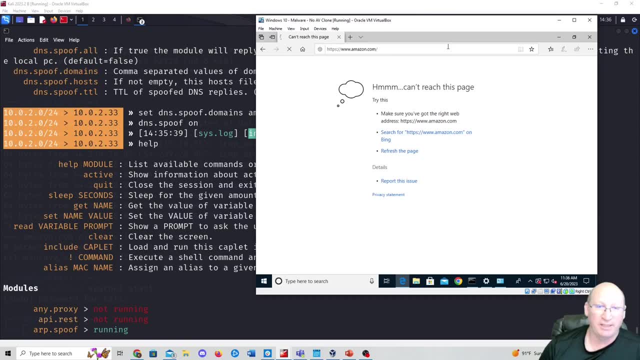 turn off. let's turn off this preferred. we're gonna obtain the DNS server automatically. let me click that press. ok, let's try this again. I'm gonna go to DNA or amazoncom. now I am seeing that HTTPS. let's do HTTP and then amazoncom, and there you go. you can see. 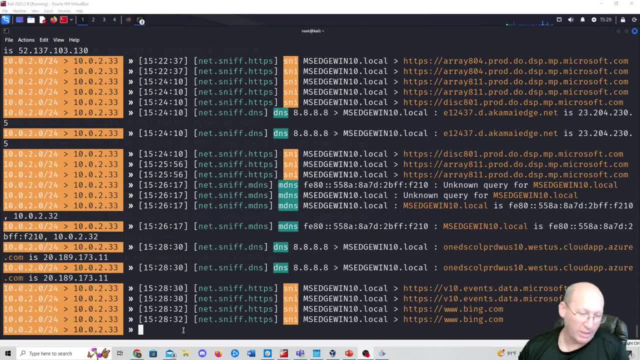 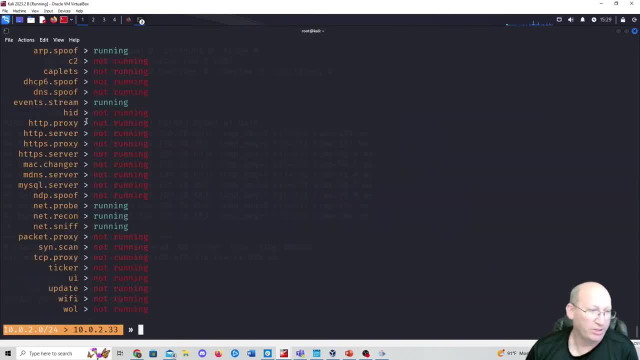 that it hacked into it now, okay. so I wanted to show you one last command before we call today. let's do that. help again, help. I cannot type today, so help. we're still running that arc spoof right here. we turn the DNS spoof off, so I'm. 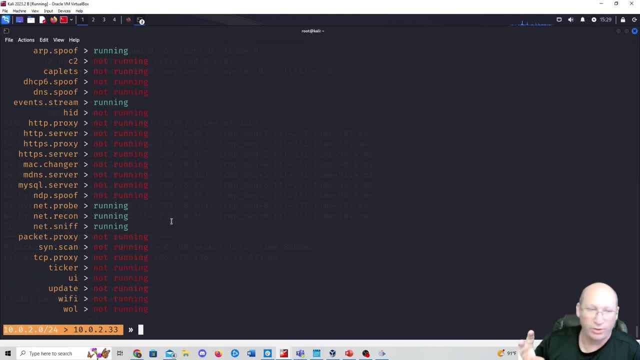 going tokhair. so evidence for this is: we're going to do an arp ban. we're gonna stop or do a denial of service tact using arp. okay, so we're gonna do ARP. let's do help first. so help arp dot spoof, just like so, and you can see that. 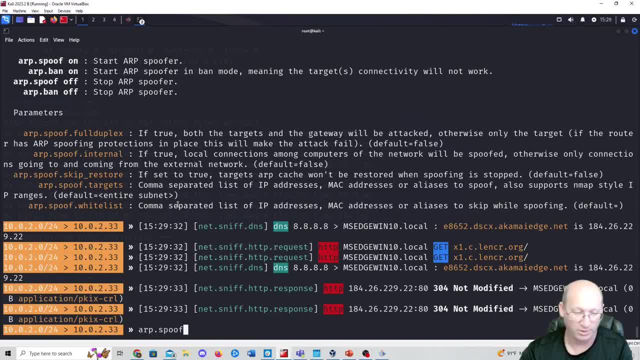 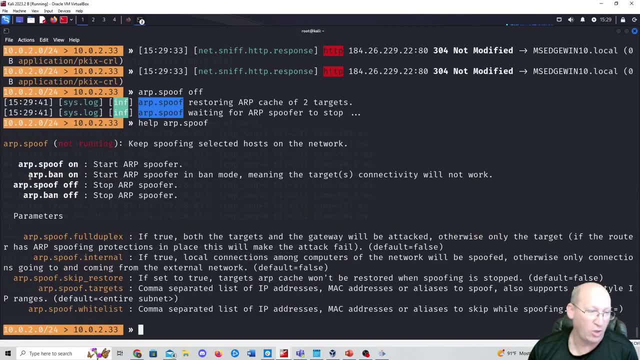 it's on. currently we need turn it off. so I'm gonna do are spoof off, so our dots spoof off and let's do that. help a command again. I'm just gonna press the up arrow twice and you can see here that I can do in our ban on right, so let's do. 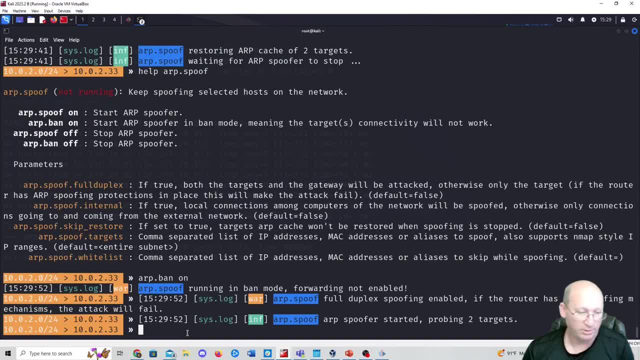 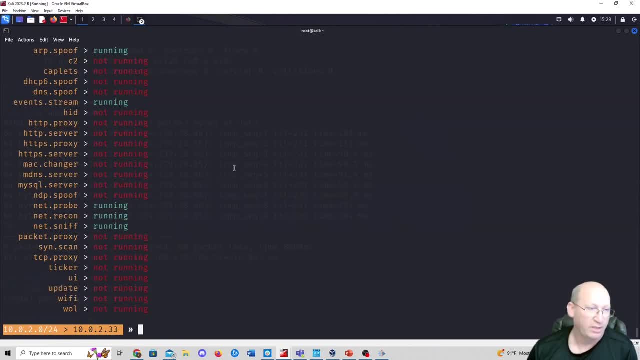 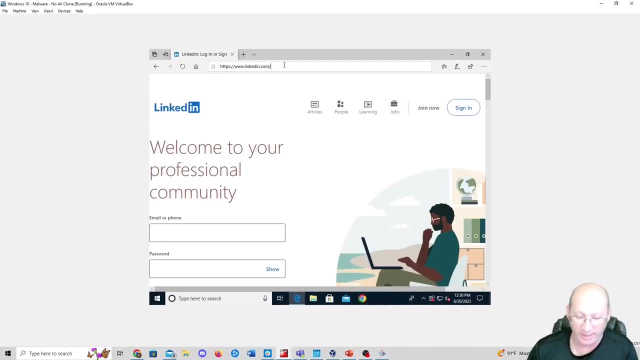 arpban on, Just like. so It's running. We're doing two targets Again, we're checking that out. I'm going to do help again And you can see now that our ARP spoof is running but it's acting as an ARPspoof. Now I'm going to go back to this Windows machine. We're going to hit a. 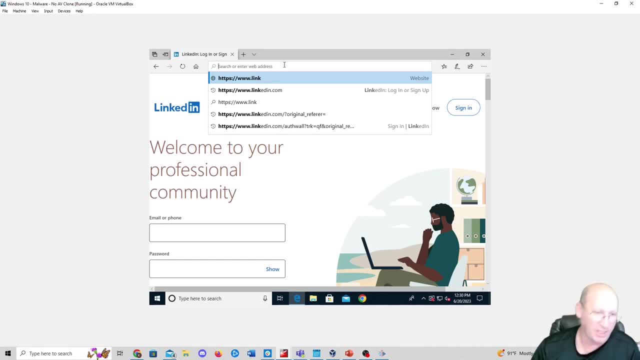 different website, a website we haven't hit yet. So we've done Amazon, We've done Google, We've done LinkedIn, Let's do Facebook. So facebookcom. And because we're doing a denial of service attack and the traffic is going through ARP but we're doing an ARP ban, it can't actually get any. 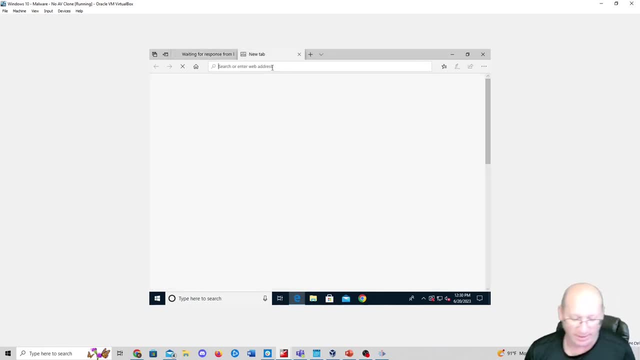 traffic right, So it's obviously not hitting our Facebook. Let's try something else. Let's try Google, Just like so, And just to make matters just apparent to everybody, let's do unicorn items, Unicorn items, And we'll hit this website as well. And you can see that they're waiting for response. They are. 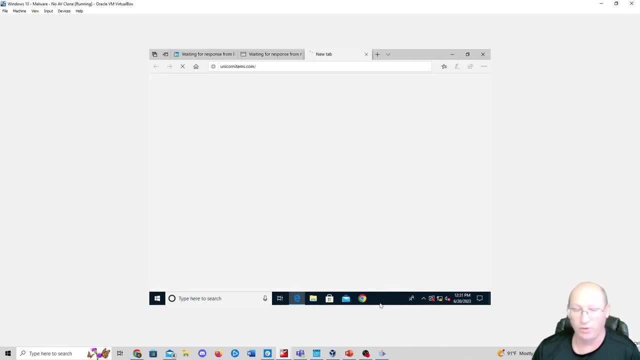 not going anywhere And that's because that ARP spoof ban or that ARPban is on. It's preventing any type of a traffic. You can even see that our network 4 is saying it doesn't have access to the network because of that. All right, So let's go back into our Kali box one last time We're going. 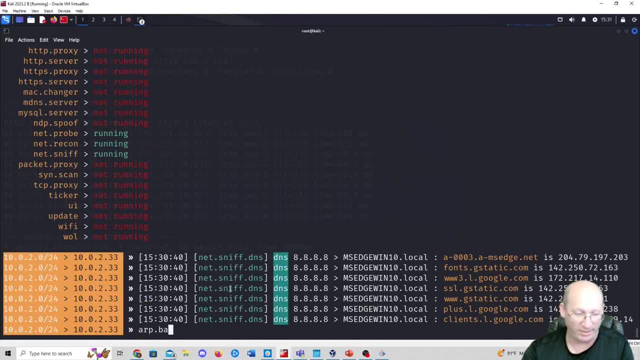 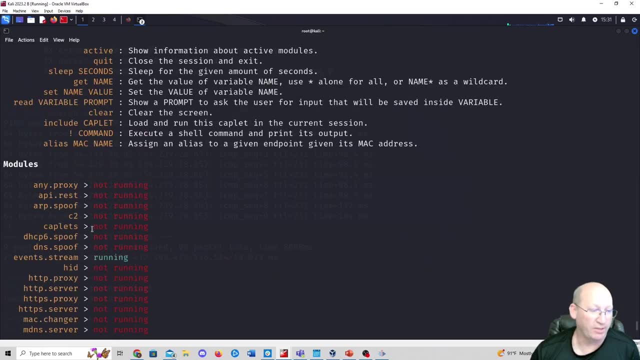 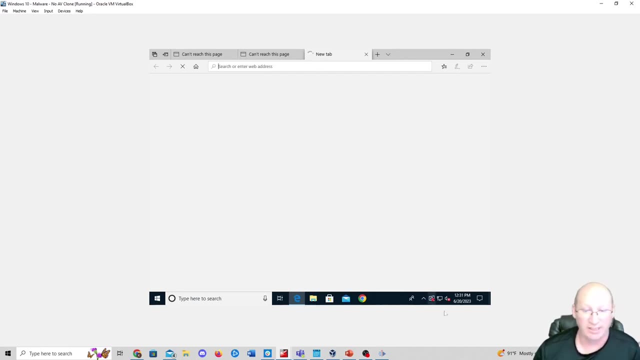 to do that. ARPban off, Like so. We'll do help. We scroll up, We don't have anything going on. And then let's go back to our Windows machine. one last, final time. Let's hit unicorn items. You can see that our internet is showing up. now, We'll do. 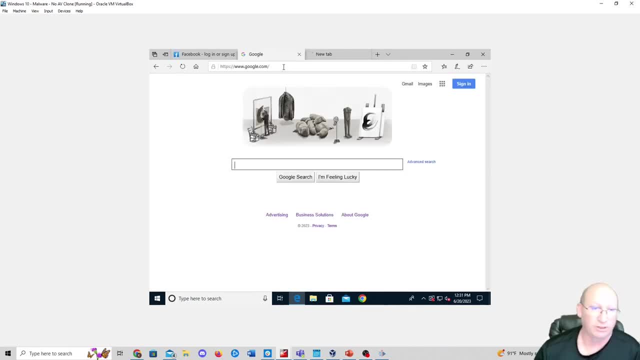 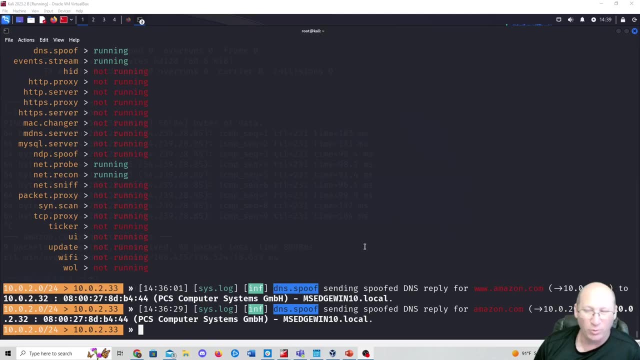 Facebook And we'll do Google Just like that, And you can see that these websites are now coming up. This is a very dependable attack that only really works if you were to invade a network in which you're kind of on a guest right. 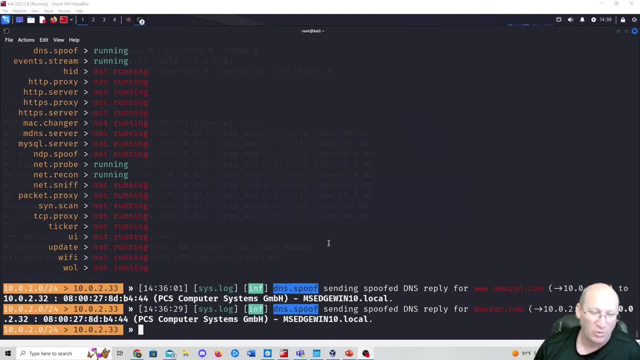 So very limited scope, but very powerful as well when you look at it from that perspective. So I hope you learned something from this. We did a little bit of DNS spoofing, a little bit of ARP spoofing or ARP poisoning and DNS poisoning. As long as we have access to this system, or as long 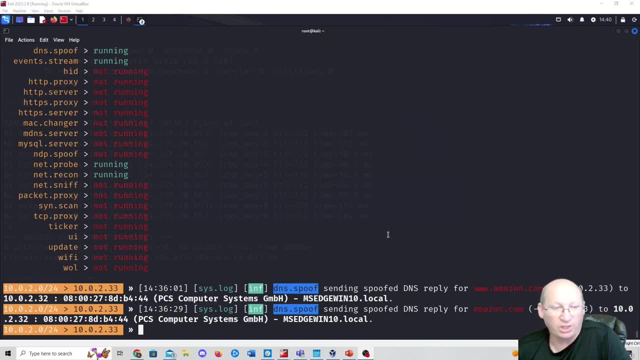 as we're inside the system with our Kali box, it'll work. Now, the scope of this attack is very, very limited, right? You have to be inside of a network. You have to have DHCP running. Your devices that are on the network have to not have a static IP address. They can't have a static IP. 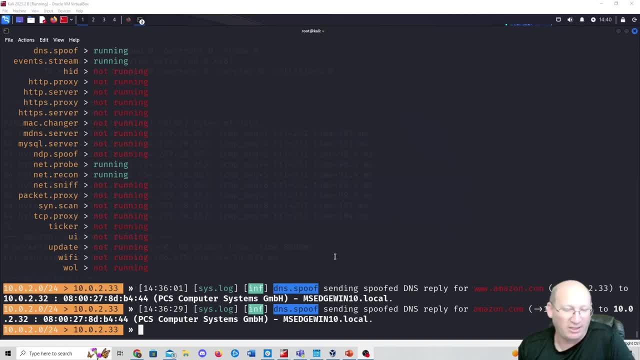 address. They can't have DNS outside of the system, And so they're relying on a lot of Fs. But I want you to think about this from a cybersecurity standpoint. How many people actually go in and set up a static IP address and set up the DNS? How many people actually do that right? And I want you to. 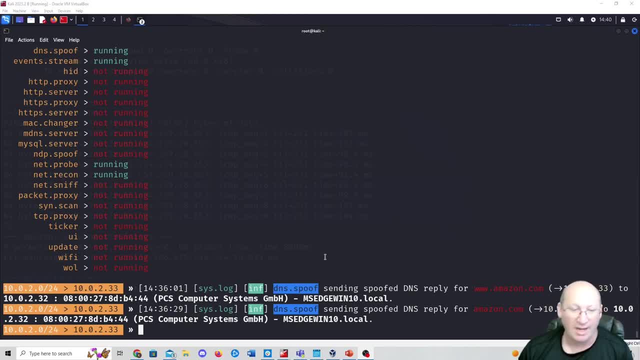 think about the same people that are using those open Wi-Fi systems, right As always. I want to encourage you to learn about this. Learn, from a cybersecurity standpoint, why it's important to protect our systems, why it's important to use static IP addresses, why it's important to have 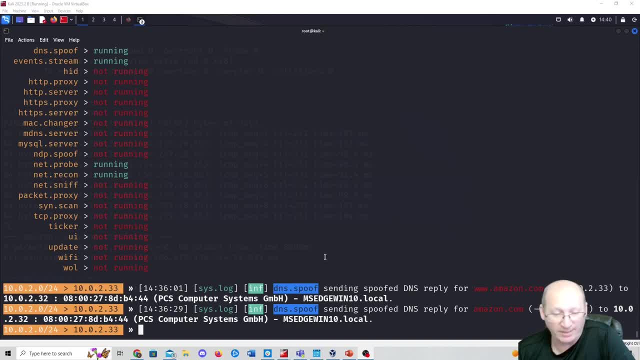 DNS set within our terminal or our endpoints. excuse me, All of that plays into the necessary part of security And, once again, don't use this in a real-life scenario. Keep it in your virtual setting. We don't want anybody going to jail. We definitely don't want to be going against the 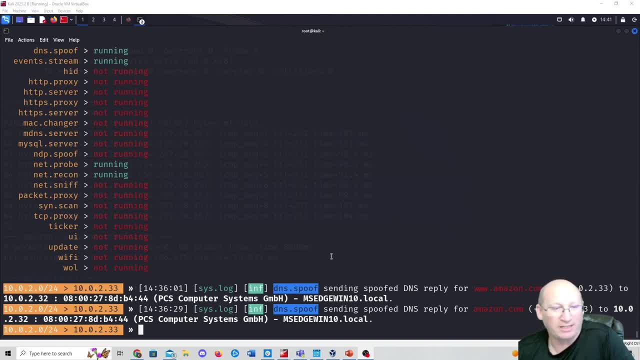 Computer Fraud and Abuse Act. all right, With that said, I hope that you learned something. If you did, please like subscribe and hit that little alert button. We will see you next time. Have a good one.